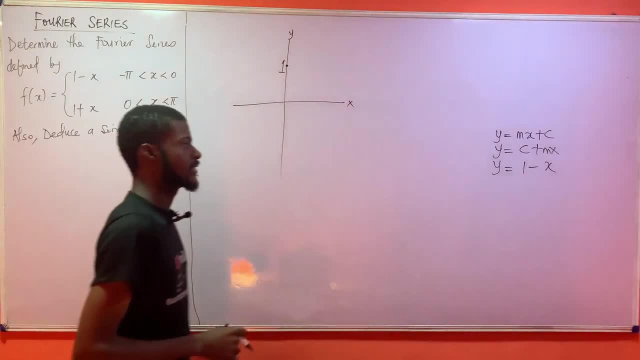 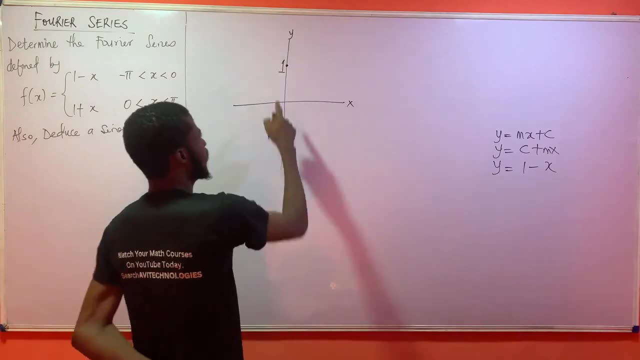 very point is going to stay, and the next thing I'm going to do is this: If this is the point, let me find another another point here. Now, what point is this? What point is this? Why is 1 here? Then s is 0, right. So this is 0 comma 1.. That's that very point. So s is 0, y is 1.. Now, what if I? 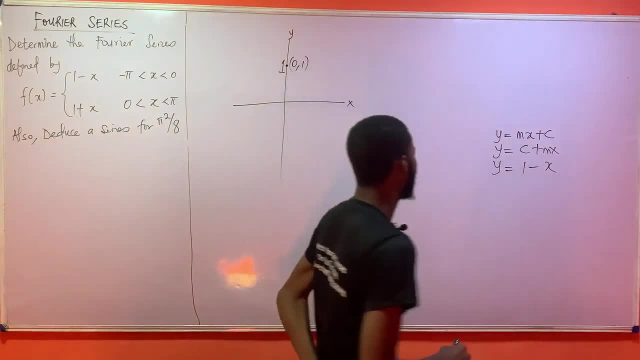 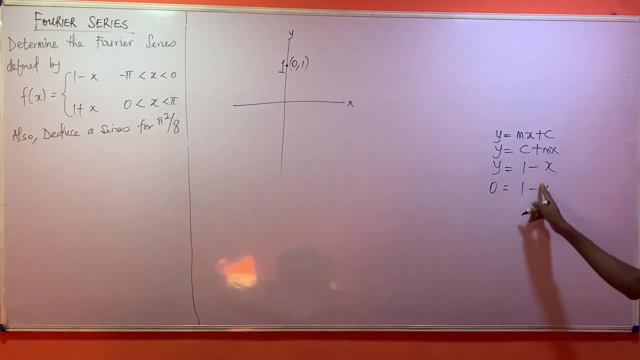 try: y equal to 0?. What do you think s is going to become? What do you think s is going to become? So? this can be 0 equal 1 minus x. Now, if minus s should come here, I'm going to have s equal to. 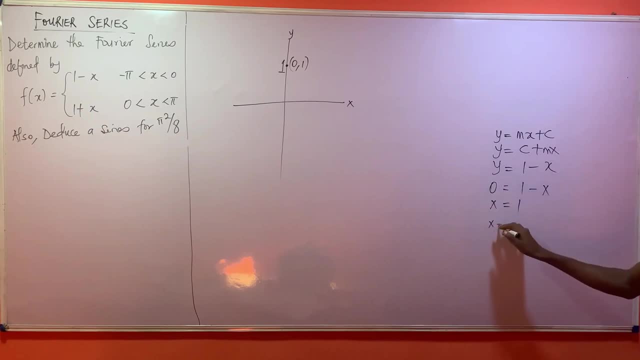 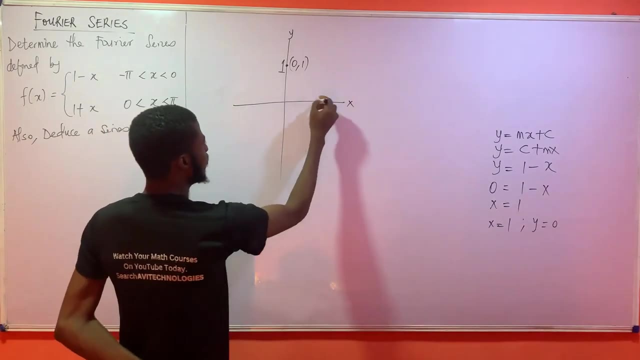 what 1.. So what does this tell me? This tells me that s is equal to 1 when y is equal to what 0.. This is a graph, right? This is a graph. We have this very graph, So let me call this very part. 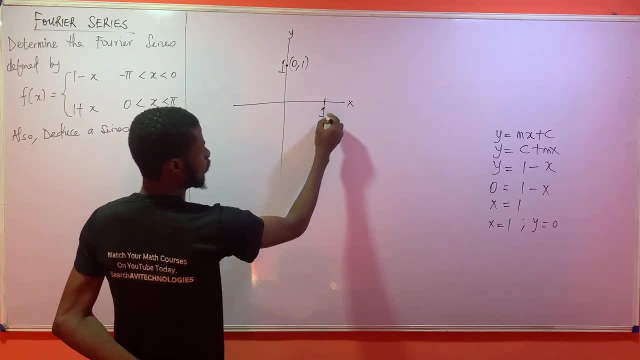 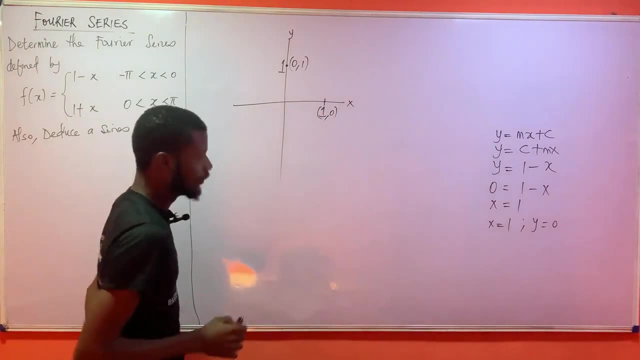 1 here. So this is a point. This point is: what 1 comma, what 0.. Now can I connect these two guys together? Yes, I can do that. Do I have a ruler? Okay, let me just do it this way with my hands. 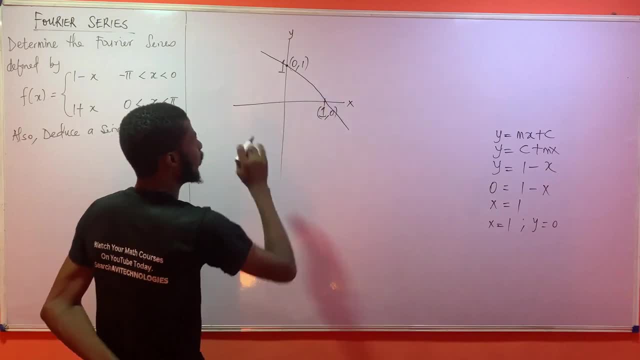 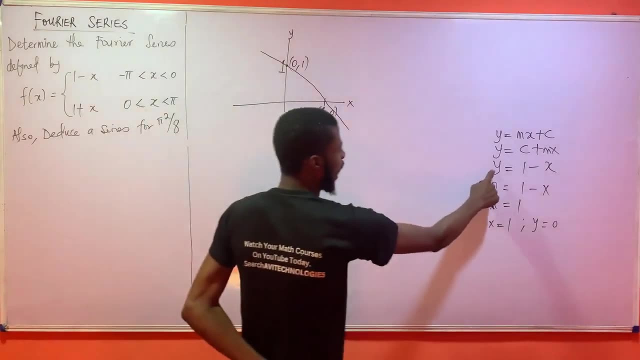 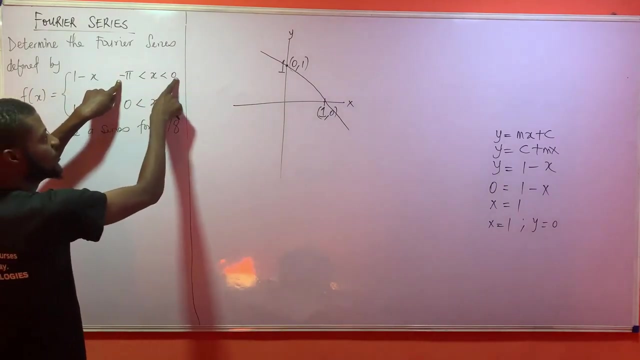 Let me just do it like this with my hands. Okay, so this is what we have. This is what we have, But listen please. The equation I am plotting is y equal 1 minus x. Okay, now what is the range of values for that? The range of values is minus pi to 0.. And where? 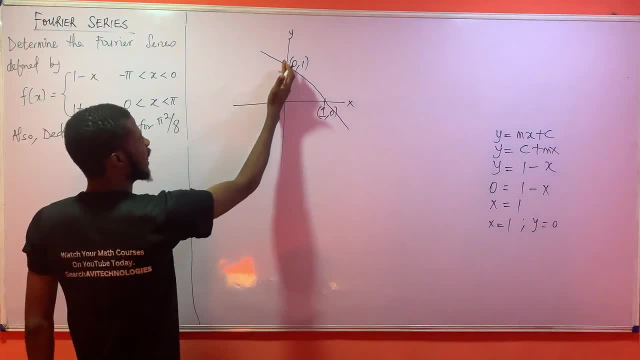 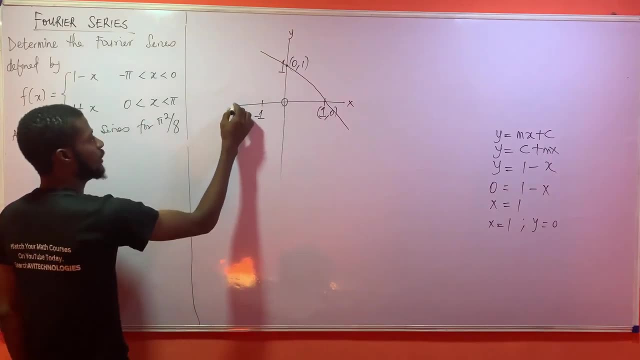 does minus pi to 0 lie? This very side? It lies at this, because this is 0.. This is, let me call this 1.. Obviously, this is minus 1.. And let me extend this and call this: my minus pi. This is 1.. Let 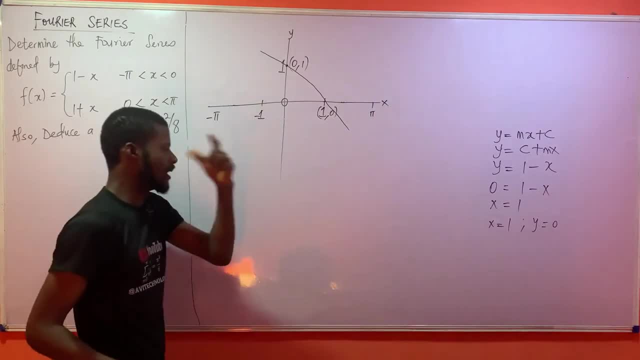 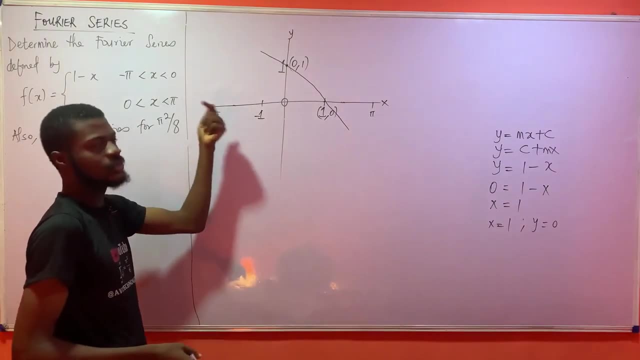 me still extend this and call this my pi, Because obviously pi is bigger than 1.. Pi is bigger than 1.. So pi is like 3.. So this minus 1 will have minus 2, then minus 3.. So that's why I am extending it. Okay, now this 1. 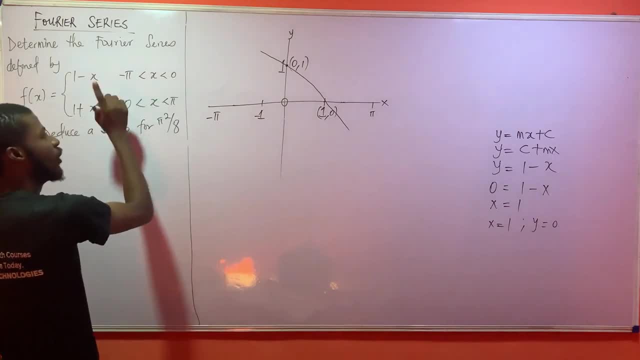 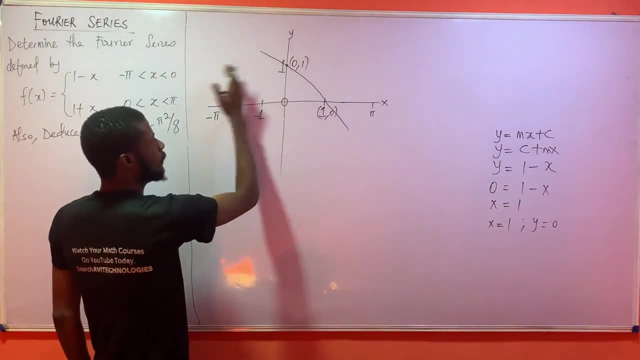 minus x that I am doing. The range of values says it is from 0 to, or let me just say minus pi to 0.. So right now it means I am concerned with this very portion. I am concerned with this very portion. So it means this line actually extends. right, That's the meaning. This line actually what? 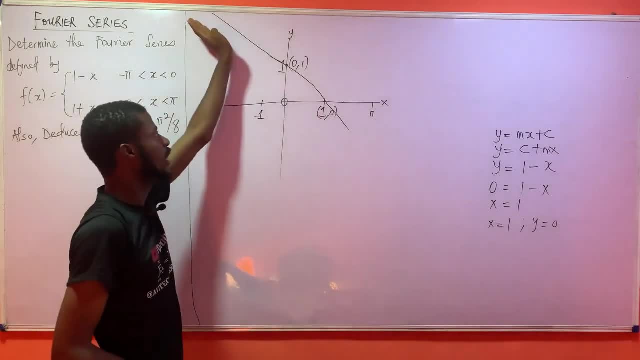 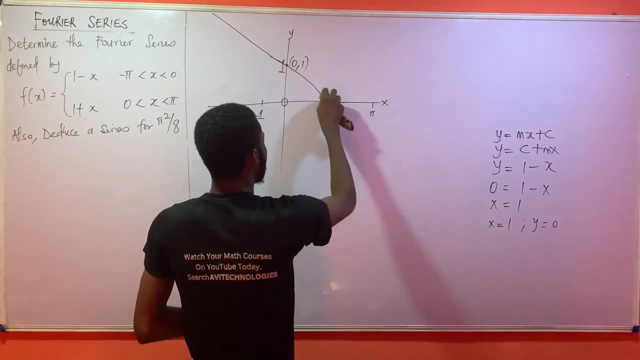 Extends Because I am concerned with this very. what Portion? That's what I am concerned with, So it means this other side is none of my business. So I am going to commut it, Though it has helped me plot the line, but it's not really important. 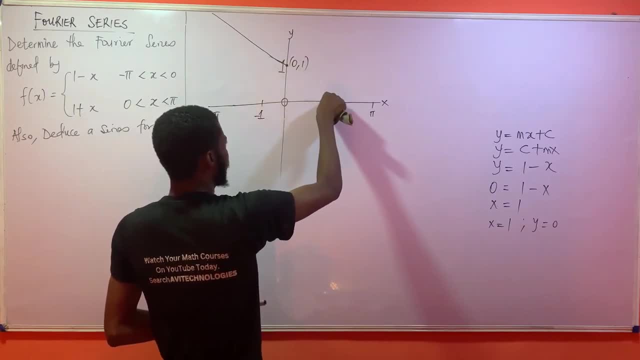 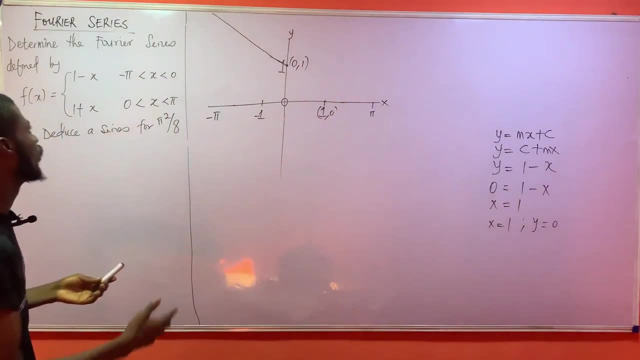 in sketching the function. It's not important in sketching the function. Okay, so this is what I have. Because why is it like this? It's very simple, Because of this very what Position I was giving to me. Now, what about this very one? 1 plus x, The same thing If you compare this very guy. 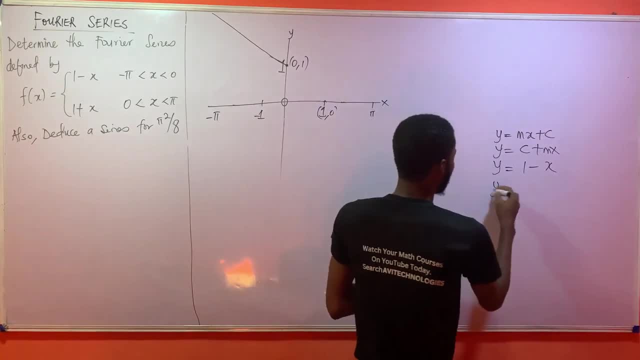 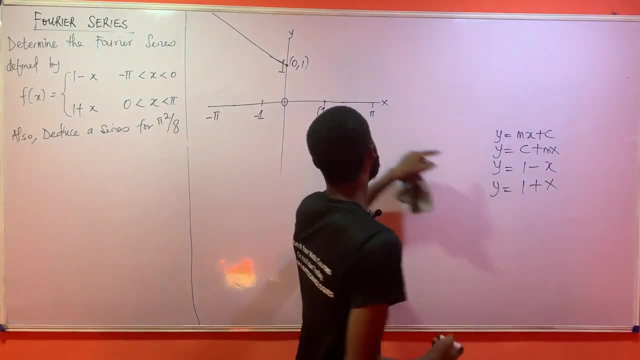 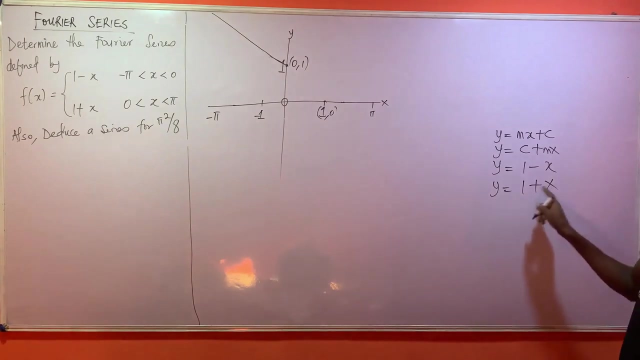 Still the same thing. If you compare it 1 plus x, You will notice that 1 here, This very one that you have here, is your intercept. So it means y intercept is still what? 1. It does not change. Now let me find the value of x when y. 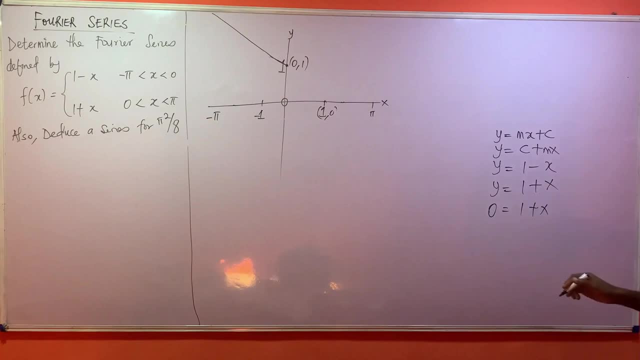 is 0.. So this is 0 equal 1 plus x. Can this one come over? It becomes minus 1 equal to what x. So what does this mean? s is equal to minus 1.. y is equal to what 0. So this is minus 1 right. 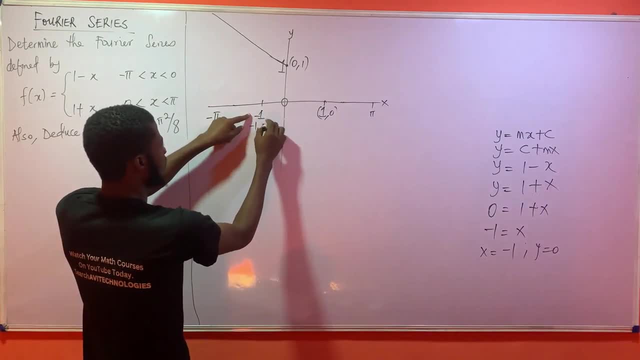 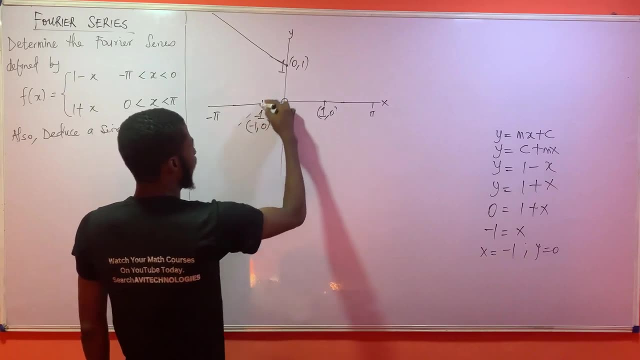 s is minus 1.. y is 0. So this guy is minus 1 comma 0.. So obviously I'm going to be drawing this very point like this. I should actually draw a line starting from here down to this very point. But 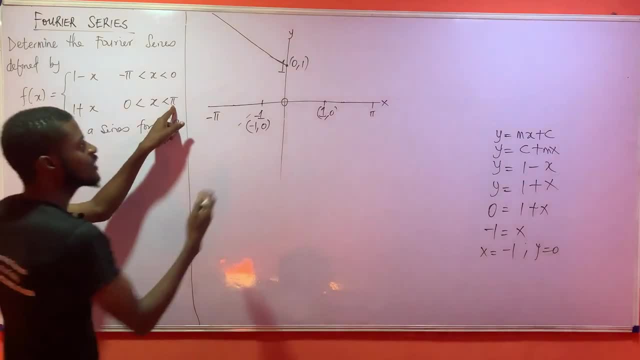 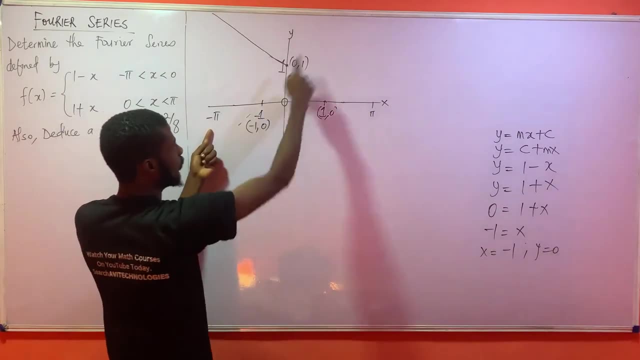 what are the conditions given? 0 to what Pi And 0 to pi is at this very location, At this very location, Not here. So it's not going to involve this negative side, Even though this line starts from here. You know, a line is infinitesimal, You can actually draw this and it does not really have 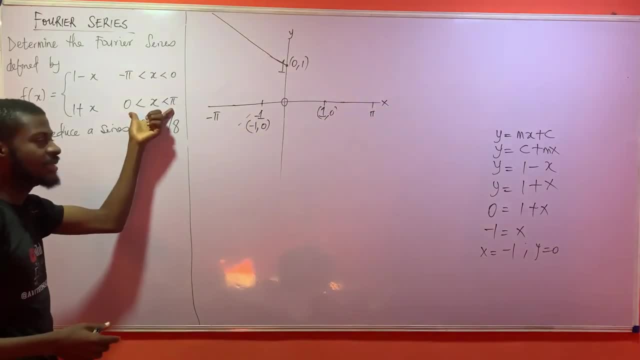 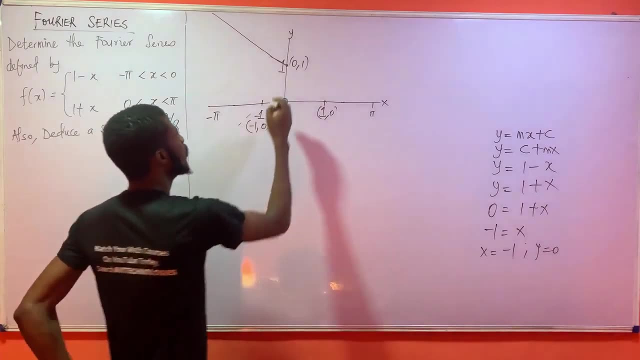 a point where it ends. But with this very guy, This very condition here, This very interval here, It is telling me where it is going to be and where it's going to stop. So that means I should take it like this: It's going this way, So this: 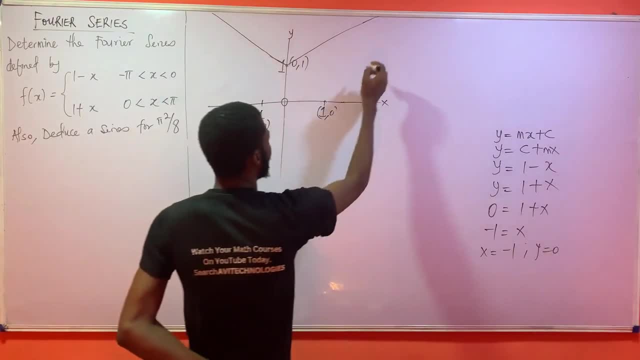 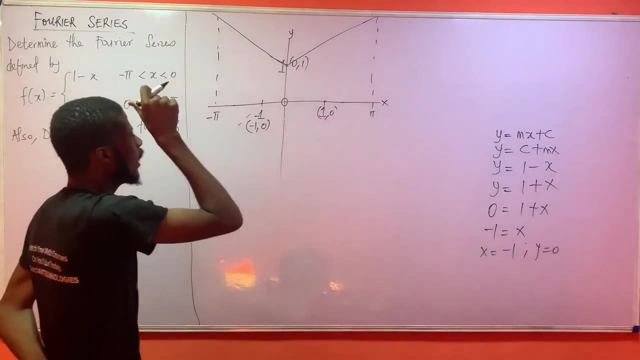 is how the graph is going to be looking like. Yes, So I'm going to trace it down to my pi. if I want to, Then trace it down to my minus pi, Something like that. Now, this is my graph, This very guy. 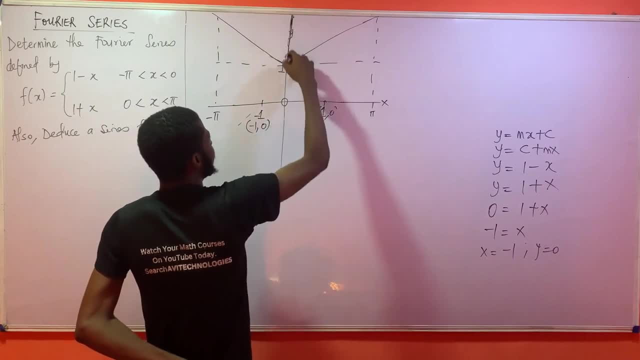 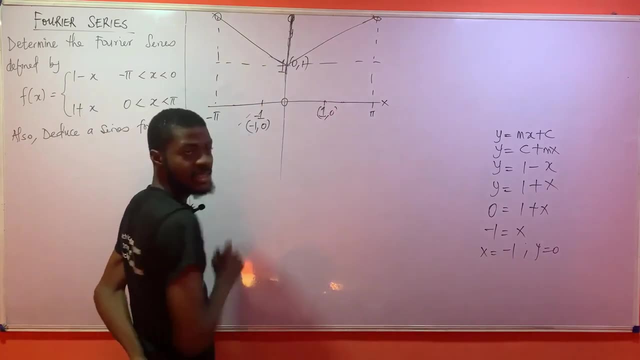 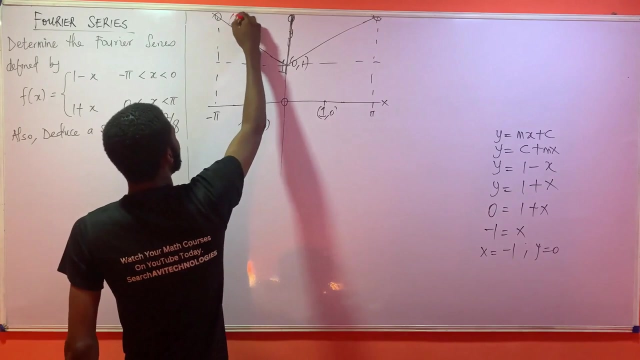 is my graph, If you notice, if I should extend y, If I should extend y from here to here, and here this guy is like half of it. right, look at it carefully please. this guy is like a half of it, if you will notice. whatever is on this very side, whatever is on this. 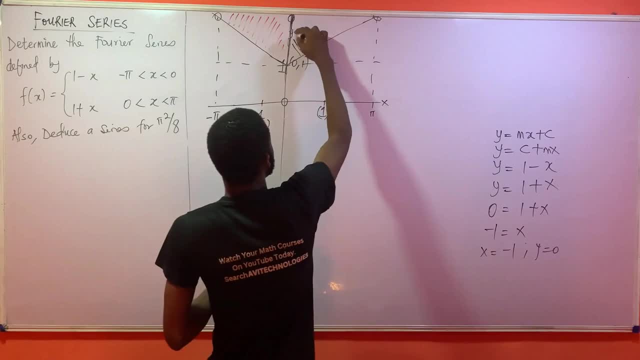 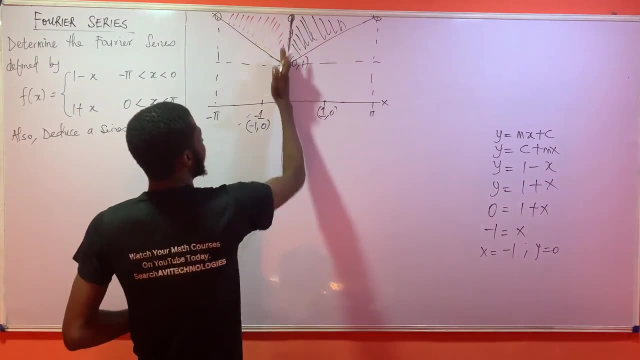 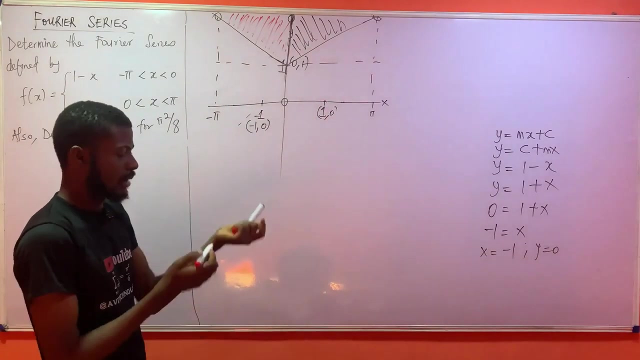 very side is actually what is still on this other side. they're actually the same. so this is an even function. because this very guy is: what's symmetric about the y-axis? this is what i have. it is symmetric about the y-axis, so this is how you will draw this. so this is what an even function. 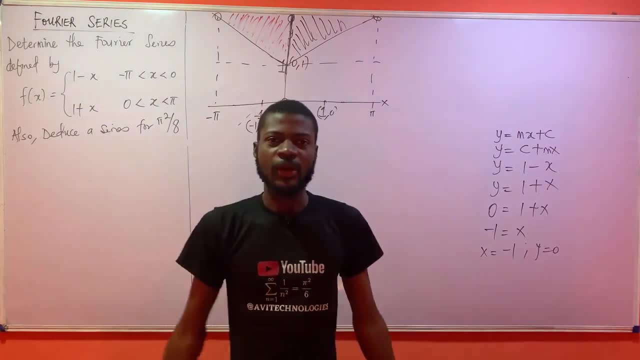 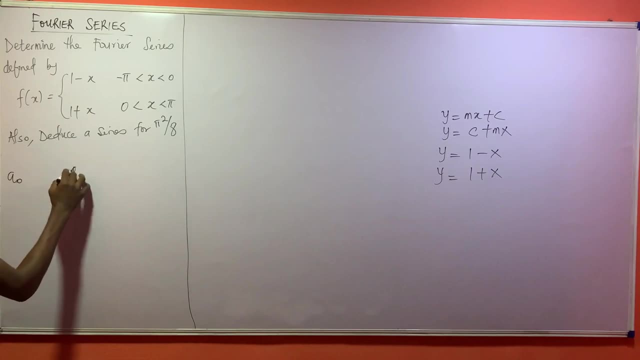 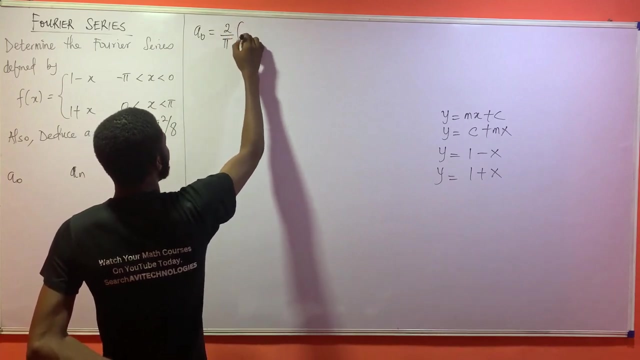 we can now proceed to find any coefficient that we need to find. so what do we need to calculate? we need to calculate for a naught and our a sub n. so let us get started with a naught. what becomes a naught 2 over pi integral? from what zero to what pi of f of s dx? 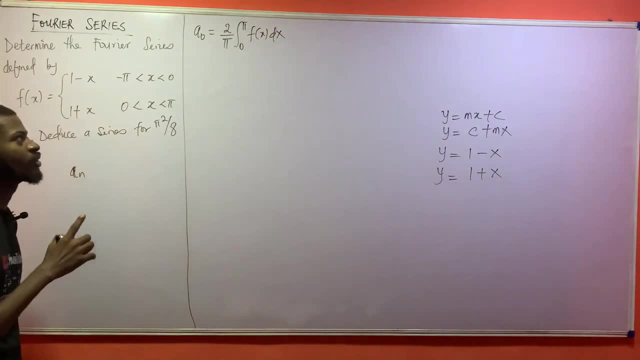 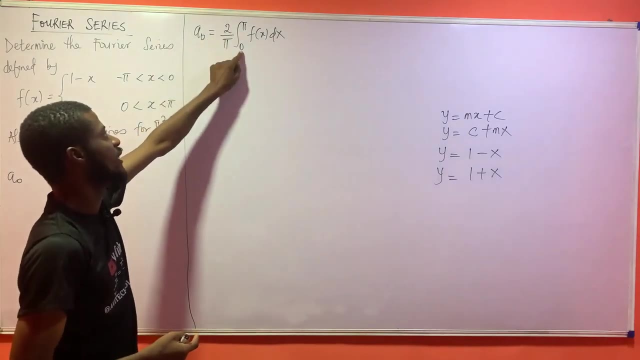 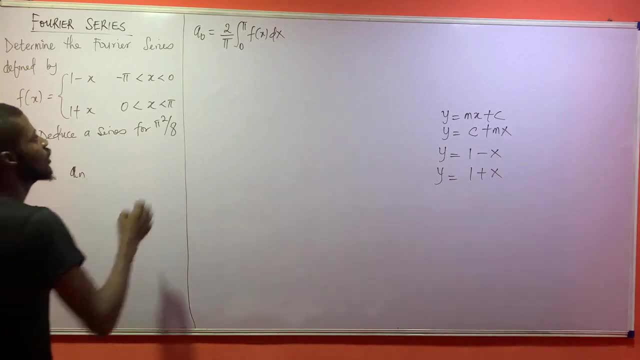 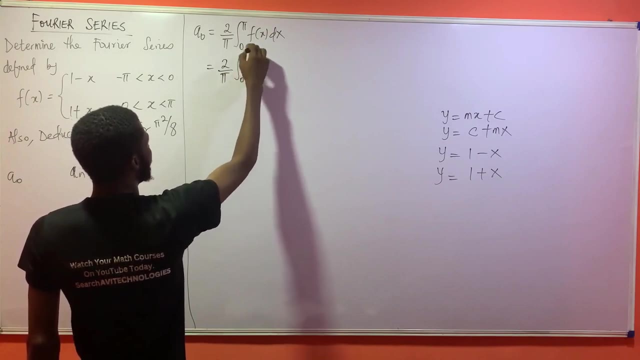 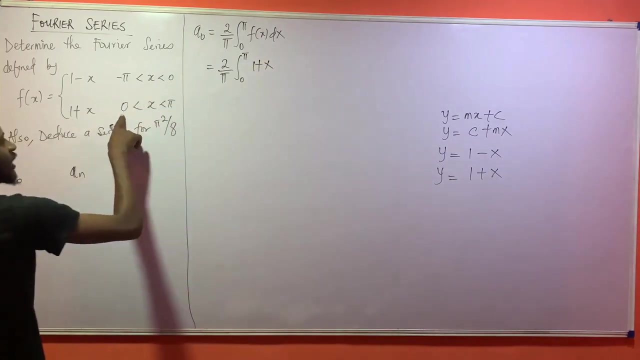 I've already explained that in the previous video. okay, so this will become equal to two over pi, then f of s. let me put my integration first of all. f of s is going to become what? one plus x. why am I using one plus s? because they said this is zero to what pi? 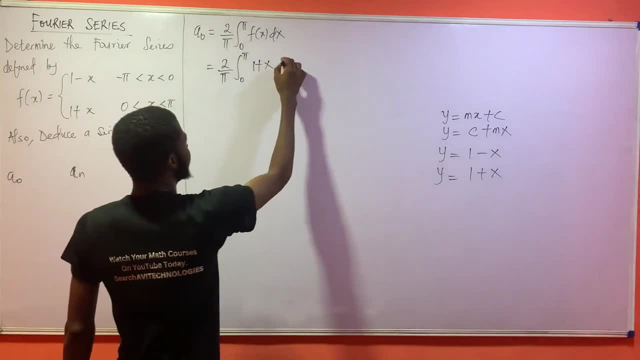 zero to pi. so I'm going to be using what? one plus x, then dx, that's something like this. okay, now do you agree that this can also be written as two over pi, two over pi? then I'm going to be having a- let me explain- bracket: integrate from zero to pi of one dx plus integrate from zero to pi of s dx. yeah, we're going to be having this. I kind of separated the one and x, separated them from each other. so this is two over pi and one dx. okay, so this is two over existence, because f of s, there's a two over myself. I'm supposed to be celebrating r straight here. so a radical我都在来. 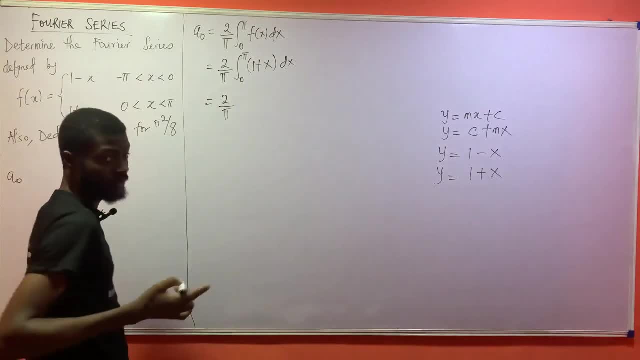 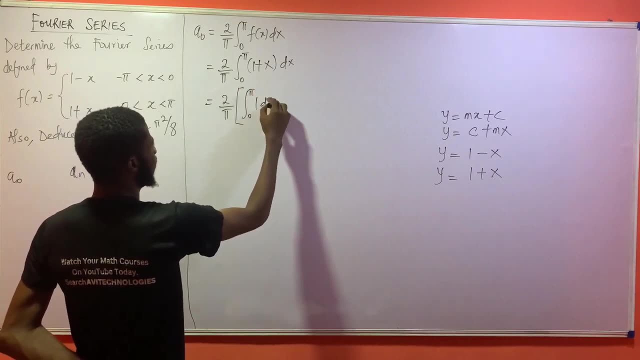 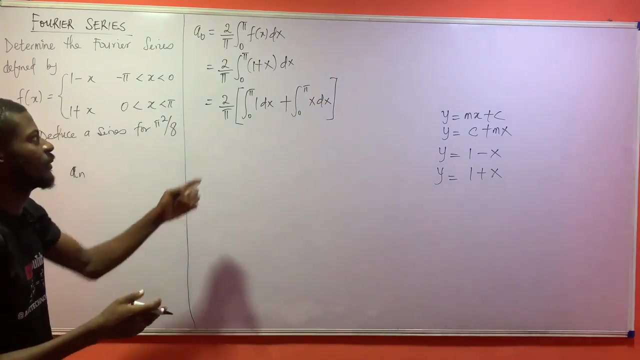 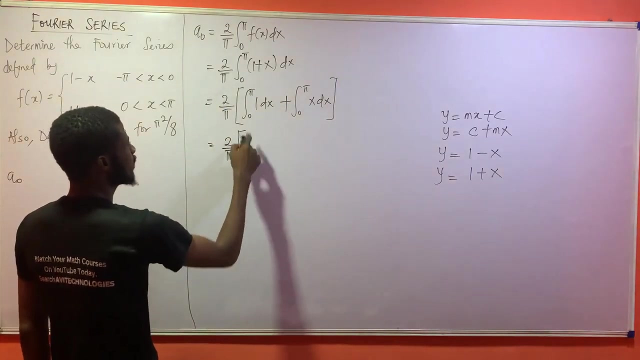 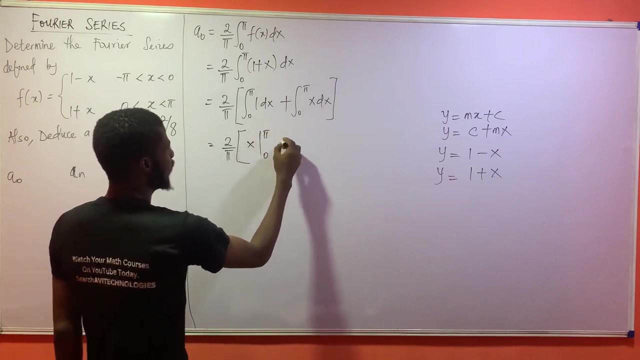 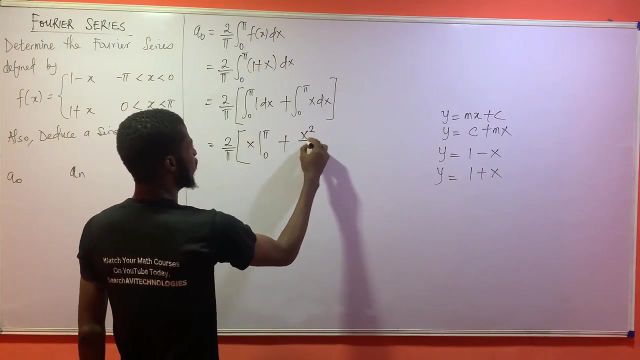 driving can open a bracket. if you integrate one, what would you get? you're simply going to get x. then put your upper and lower limits zero to pi. then, plus this very guy, if you should integrate x, what are you going to be having? you'll be having s squared over two. you know. 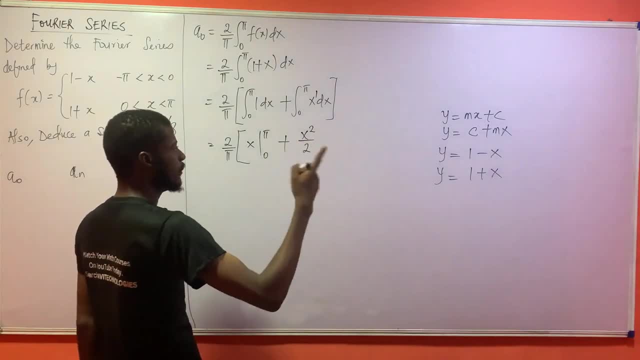 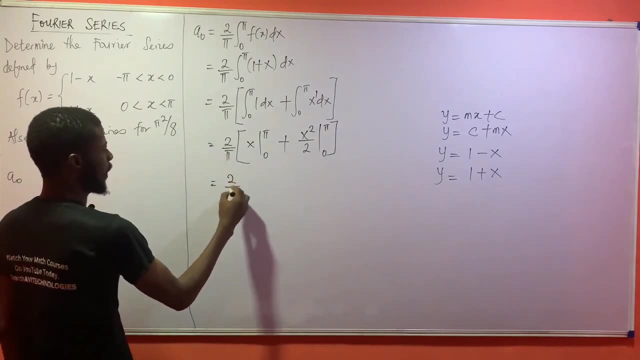 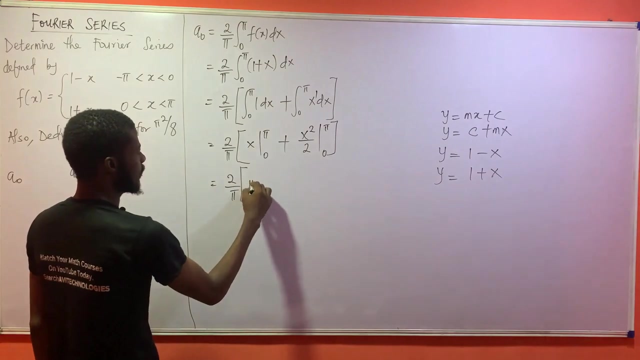 this is a one, right. you're going to say one plus one over one plus one, okay, and then you put your lower limit zero towards pi, okay, and this will become two over pi. then let us put this guy together. remember what am i going to do here? i'm going to say s should become pi, so this is pi. 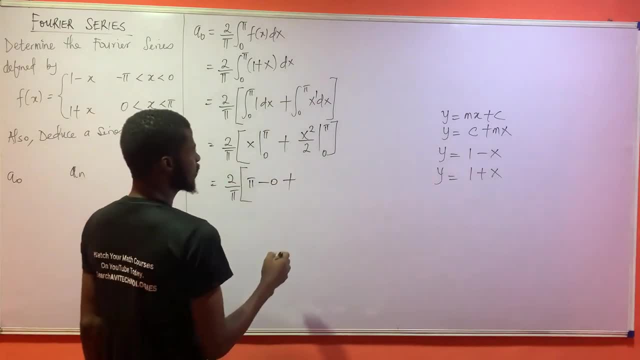 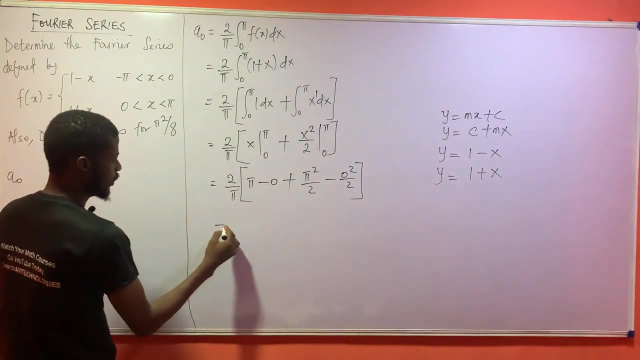 minus s is what zero. then plus all. i got this very side. i'm going to say s will become pi. this pi squared all over two, minus what will s become zero. so this is zero squared all over two. what i just did is very, very easy to understand. so this is two over pi. then pi minus zero is pi. 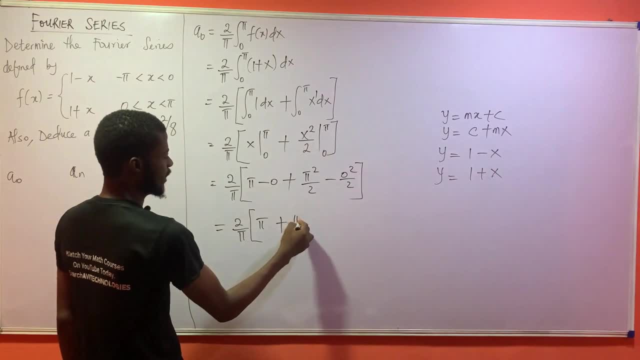 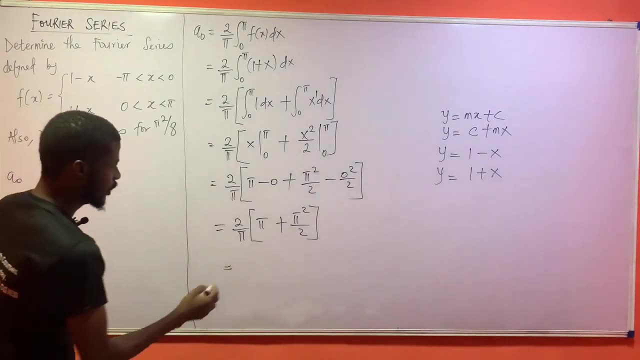 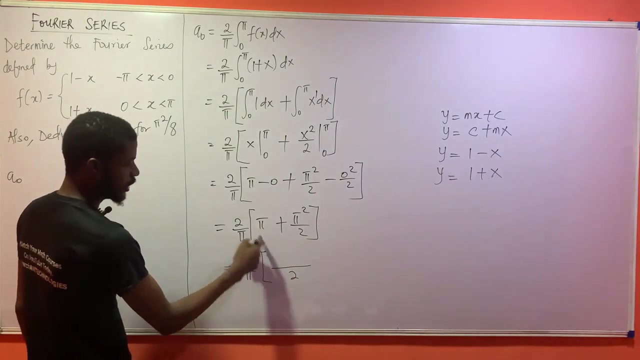 plus, this guy will become pi. what pi squared over two, because this part will become zero. okay, now look at this properly. this is two over pi. we have two over pi, um. i can say. i can say that, um, let me open a bracket. what is the sm of these two guys? two, so two times. this will give me what this will give me: two, um where. 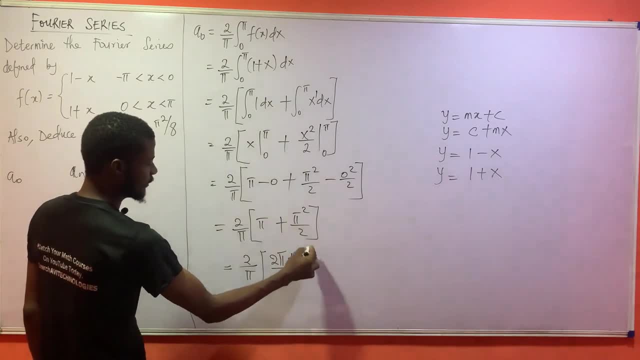 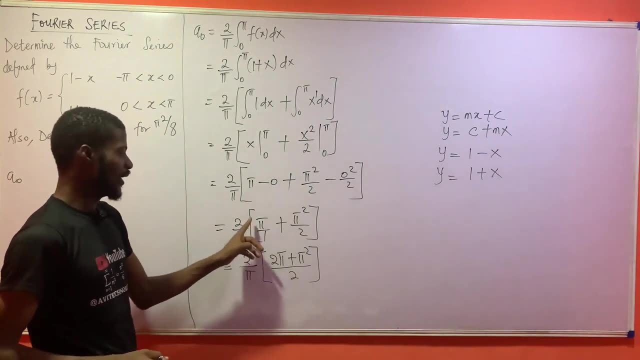 is this guy two pi plus pi squared. look at it here. this is actually one right, so two times sorry. two divided by one is two times pi is two pi. then two over two is one one times pi squared is what pi squared. now i can first of all say: 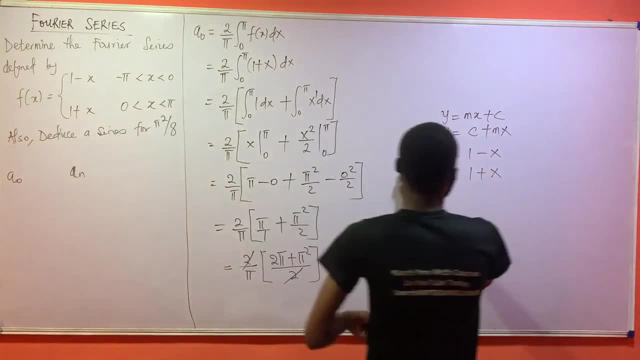 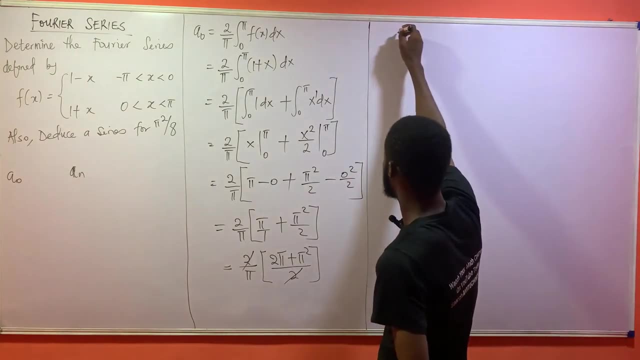 two should cancel two, like let me just do that first of all, so i know where i am at. okay, if i should proceed with that, i would then be having this to be equal to, if i look at this properly. if i look at this properly, all the left to become 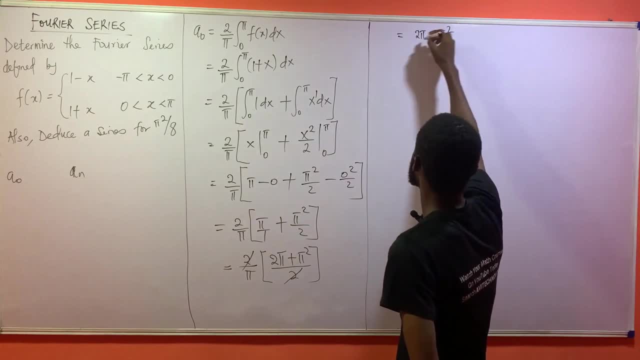 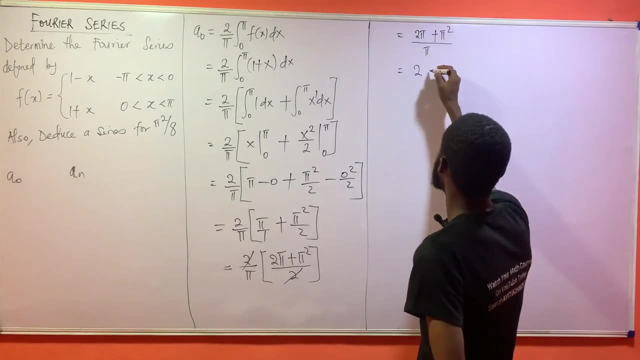 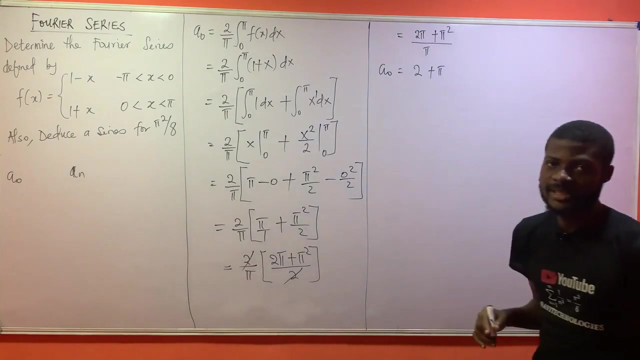 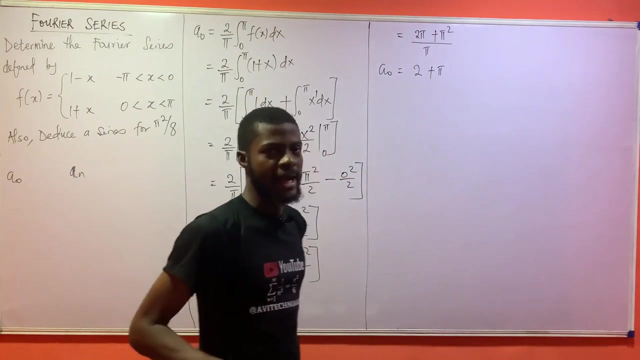 two pi plus pi squared everything over what pi. now this become two pi over pi is two. right, we have two then, plus pi squared over pi is what pi. so it means your a naught is equal to this very guy. that's the meaning. so this is your a naught, this is a naught. so we have two plus pi as our a naught. 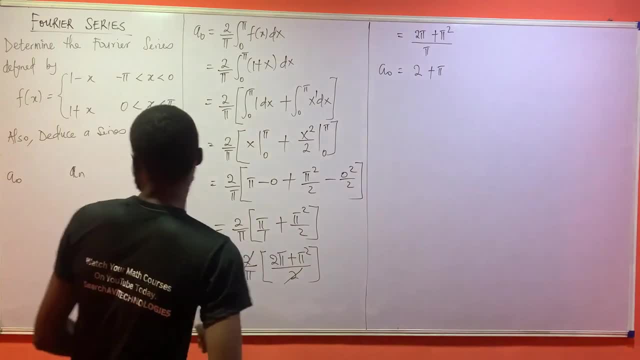 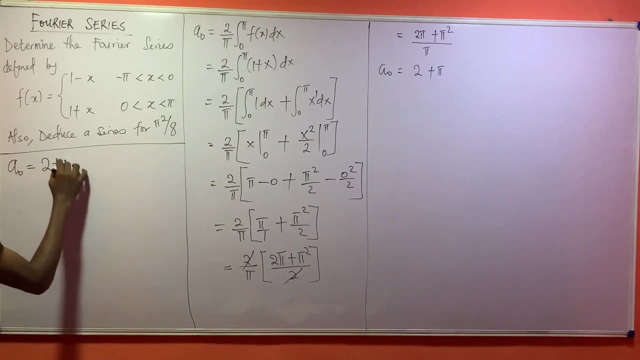 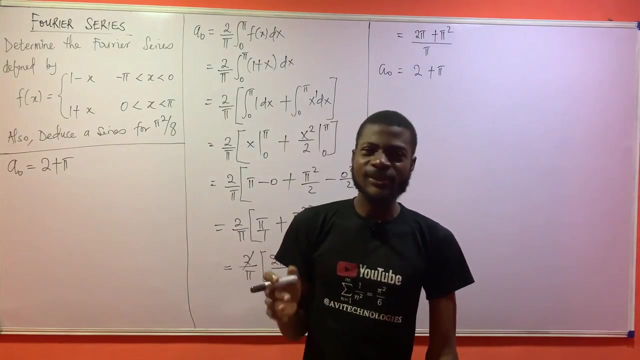 so you keep that somewhere. keep it somewhere, so that's our a naught. let me even write it here. let me write it here. so a naught is equal to plus pi, so that's a naught. now, if you've stayed up to this part, please, i want to beg you guys for something. i noticed that girls are not really 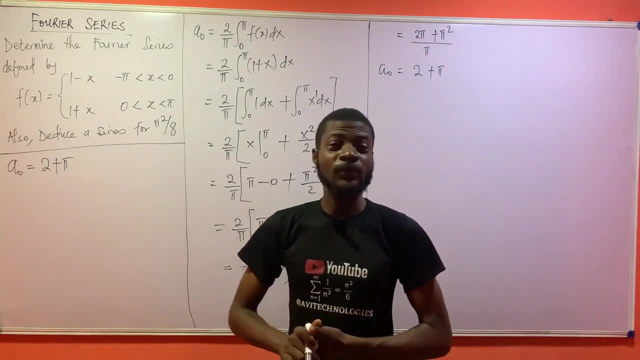 watching my videos. i don't know why, but youtube clearly tells me that the percentage of males watching my videos are 100 percent. i don't know where we have females in engineering right, so please share this video to your female classmates. thank you. okay, so a naught. 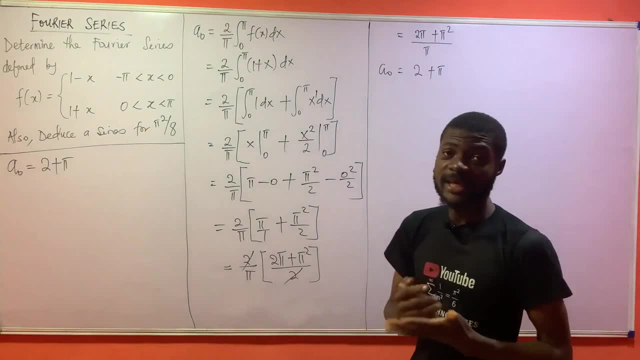 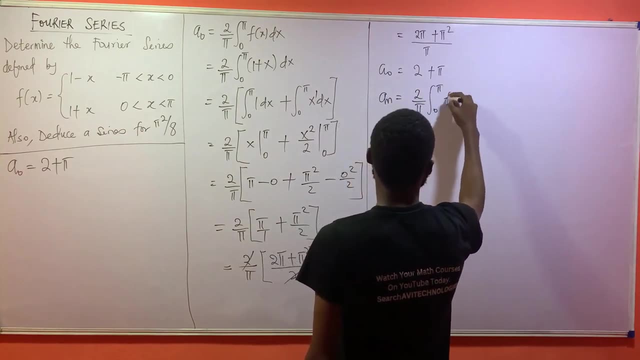 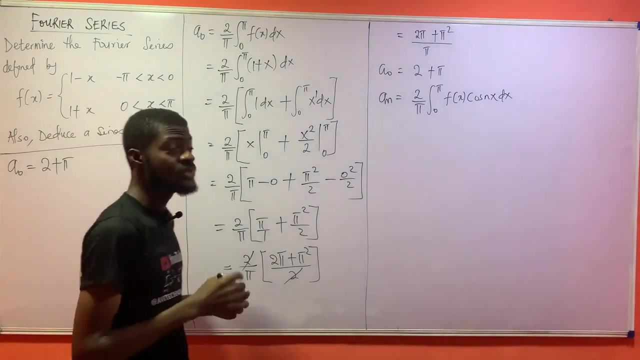 is equal to two plus pi, but the next thing i'll find is my a sub n, now a sub n. the formula is: two over pi, integral from zero to pi f of s, cos, nx, dx. okay, so that is your. this is a sub n, now why is it? 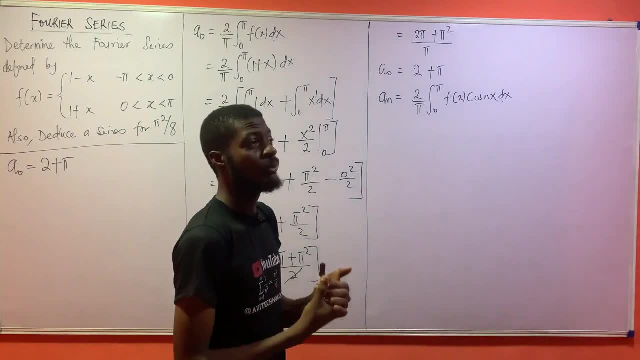 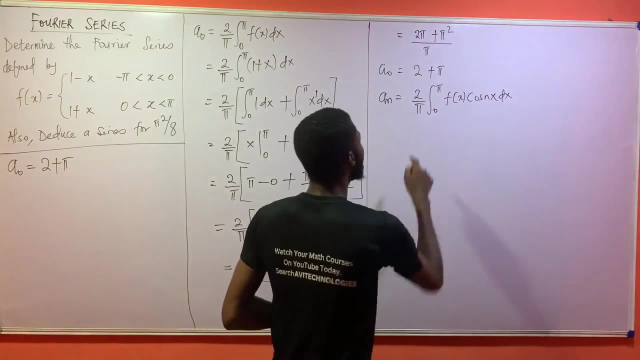 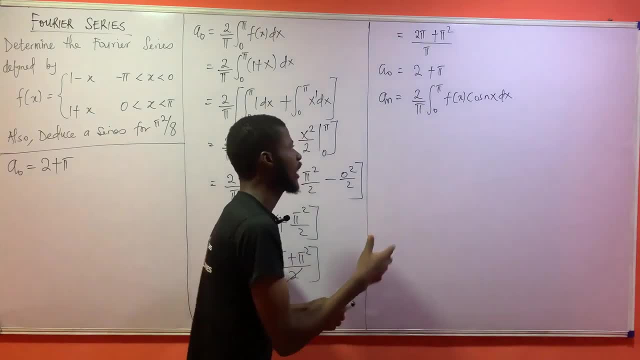 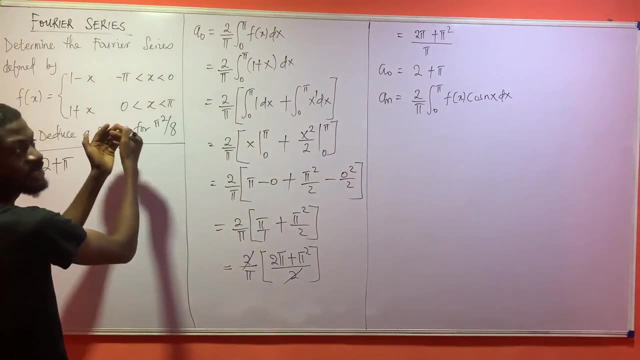 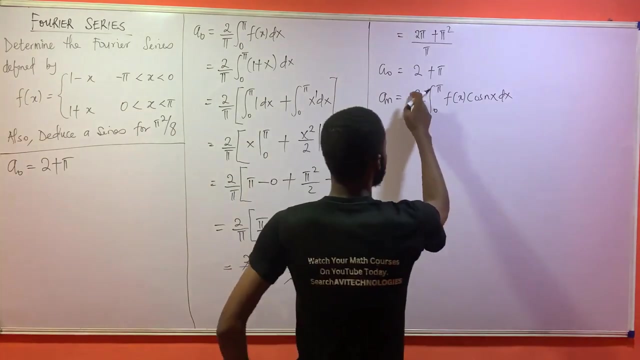 two is a two here because it's an even function. so i can actually reduce this part, this very interval, to this interval. they are symmetric, so i can just pick one part of it, get the value of times it by two. so i'll just integrate the two without me wasting time, okay, so that's why this. 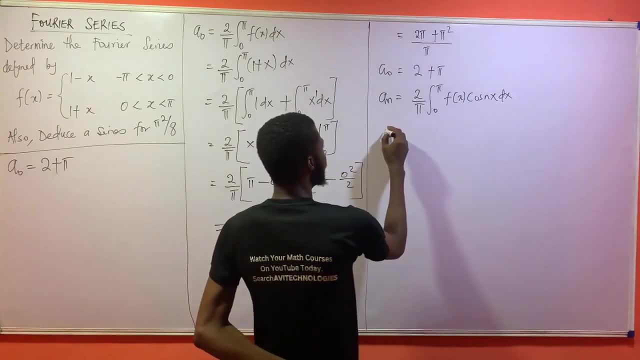 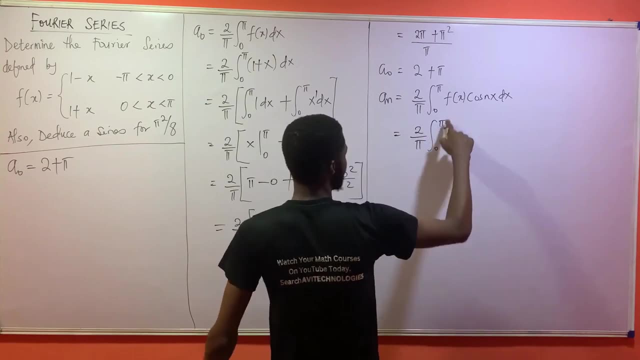 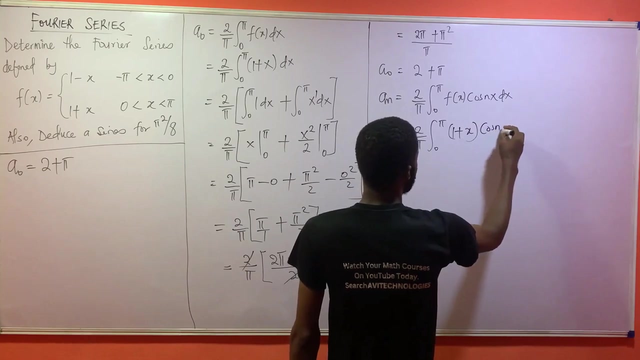 two is here to understand more, watch that very video. so this is a sub n equal to over pi, integral from zero to pi. which of the functions has zero to pi? this very guy is zero to pi. so this is a sub n zero to pi. so this will become one plus x, bracket, bracket, cos, nx, dx. this is going to be very, very. 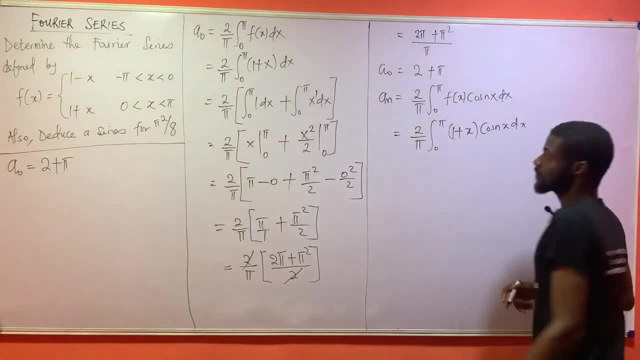 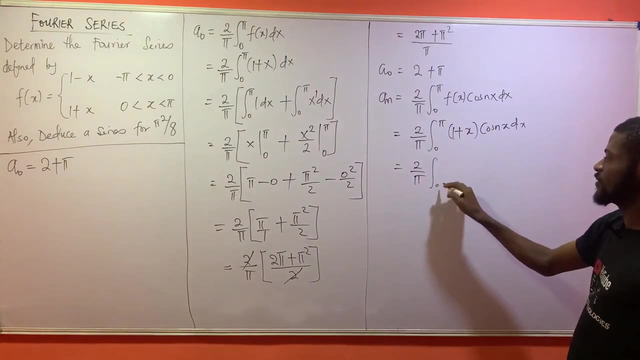 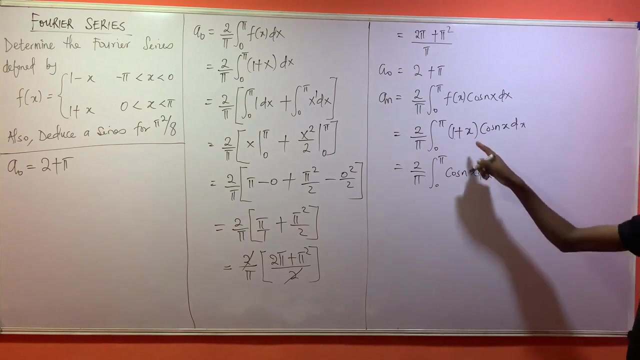 very, very beautiful for us to integrate. okay, and let us see, this will become two over pi, um, okay, integral from zero to pi. one times cos nx is, cos nx dx, then um, i have plus s times cos nx ns is, is cos nx then dx? okay, remember that this is going to actually be in a bracket. 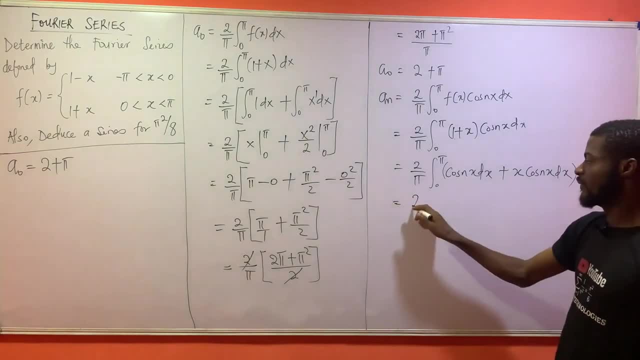 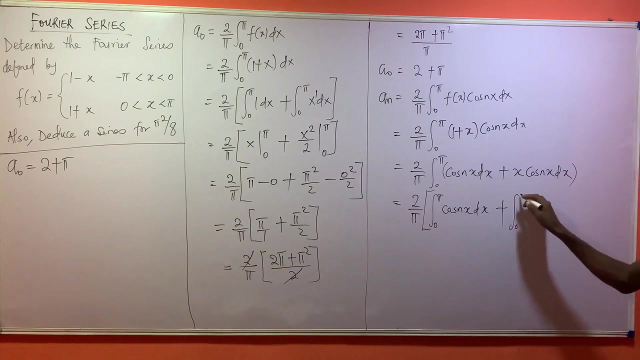 because i still have the integral sign here. now this is 2 over pi. can i do something here? can i say this is a bracket, integral from 0 to pi of everything here, cos nx dx, plus integral from 0 to pi of this guy s cos nx dx. 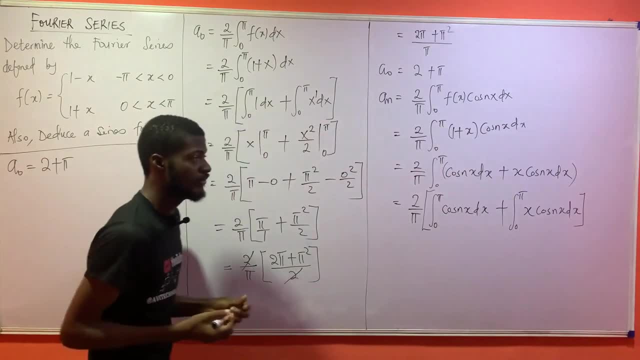 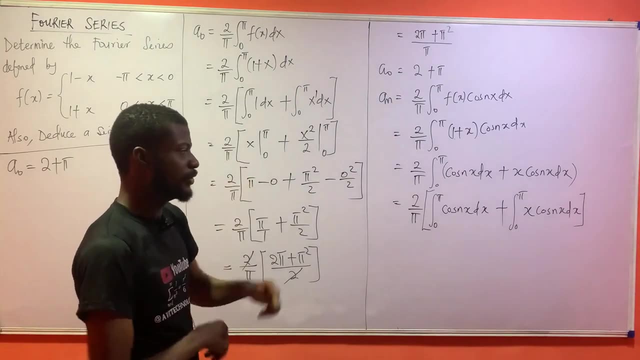 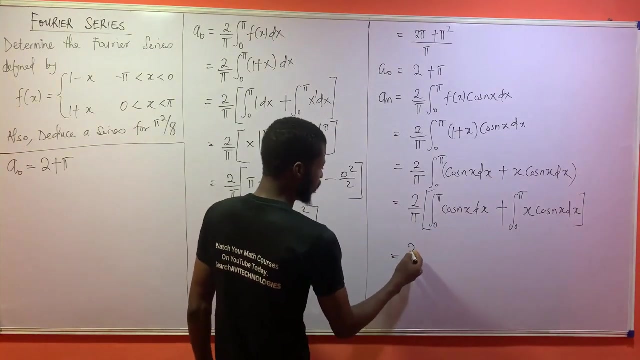 i can do this. it's possible for me to do that. it's very, very possible, okay, so this is what we have. this is all we have. that's what i'm going to do here. i'm going to proceed. i'm going to integrate each of them, so we're going to start with this very side. so this: 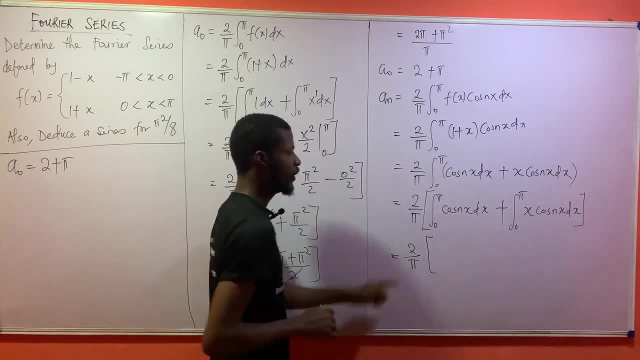 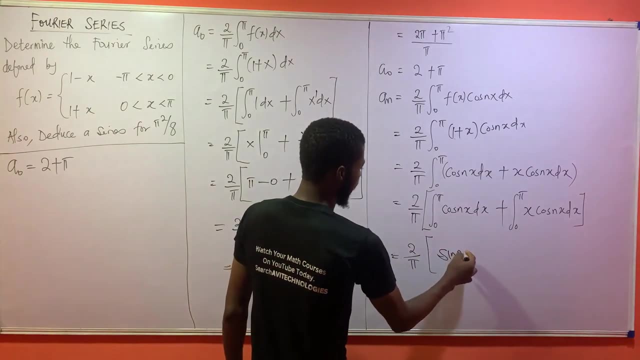 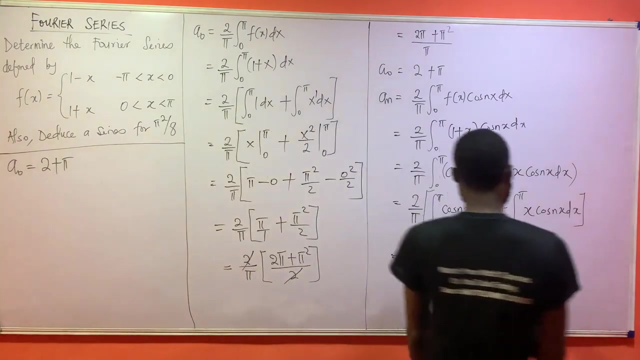 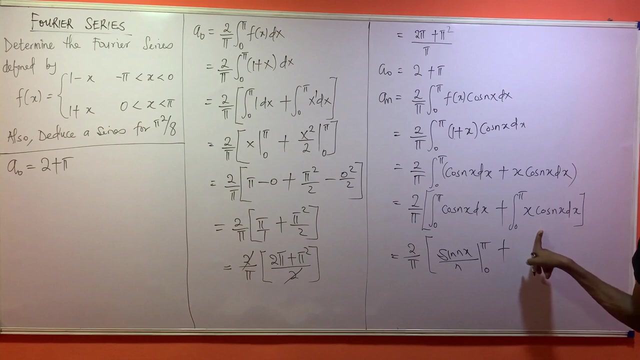 2 over pi, um, open this very guy up. if you should integrate cos, what would you get sine? so this is sine: nx over n. from what zero to what pi? because we're going to put the upper lower limit then plus. if you look at this side carefully, you look at this side carefully, this is going to be solved. 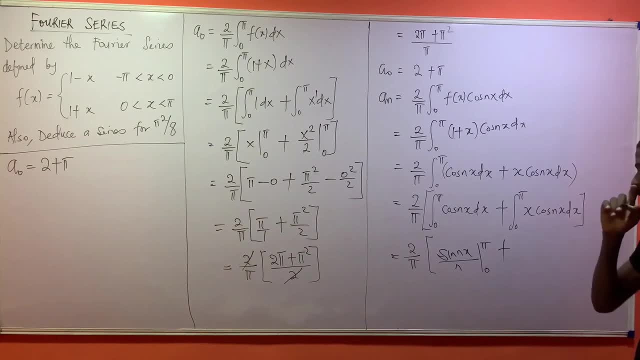 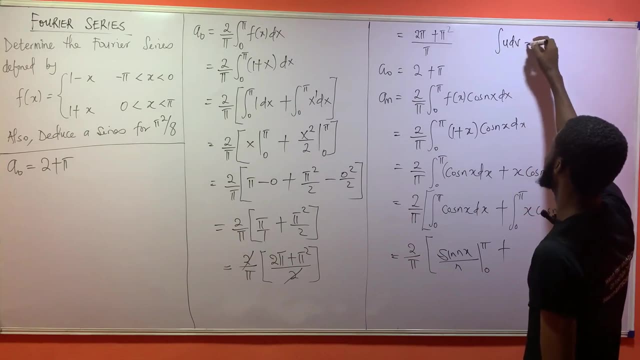 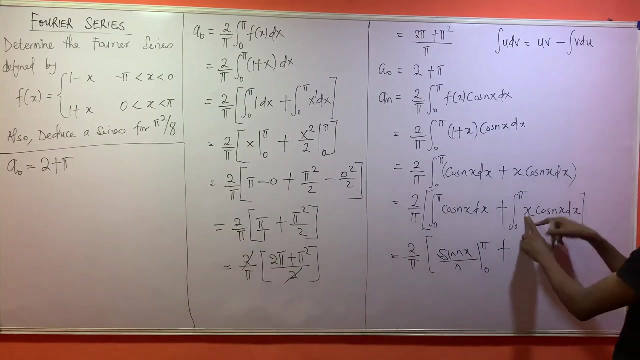 using integration by parts, because i have two products here. so i'm going to say let this first guy become u. let's become you. remember that the integral of u dv is equal uv. take away integral of what vdu, if you can remember. so let me call this very x, my u. so let's u equal to x. then um dv. 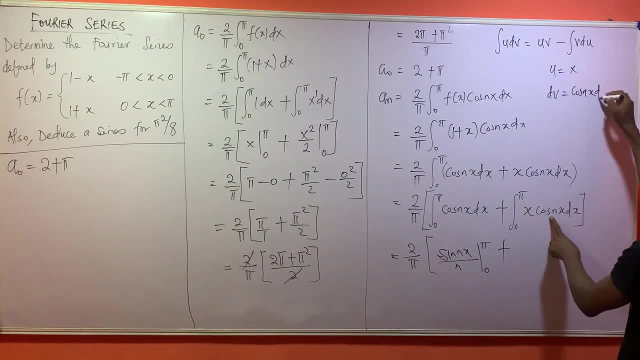 should be equal to what? cos nx, dx. so that's what dv is going to be. now, if u is equal to x, what do you think du is going to be? d is going to be what come what one? because if we should differentiate x, we're going to get one. dv is equal cos nx. how do i get my v? because it's dv, so to get. 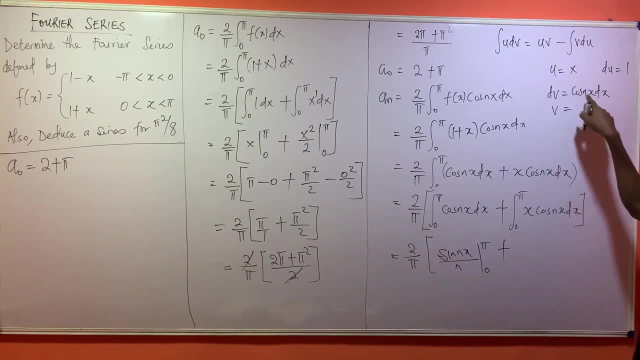 your v. they're simply asking you: what did they differentiate to get this? so you simply do the opposite, which is integration. so integrate this all you get. you're going to get sine nx over what n? yeah, something like this. so that means i'm going to say, using this very formula, i'm going to write: 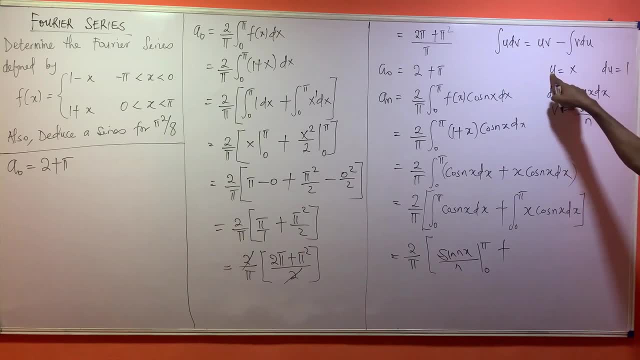 uv. so where is my uv? this is u, so this will become u, which is x. then this very guy is sine nx over n. just then the limit is zero to pi minus minus integral. from zero to pi again, um vdu, what is our v? v is equal sine nx over n. okay, yes, then um du is equal one. so i don't put dx here. this would be. 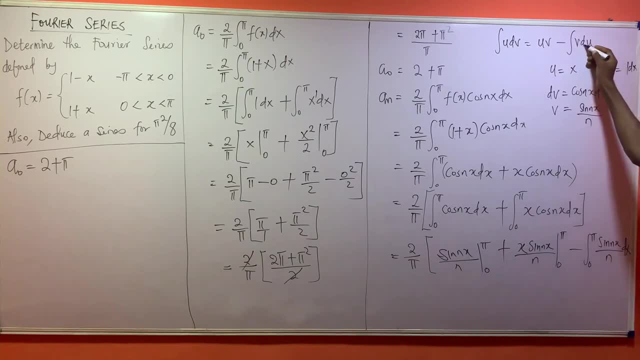 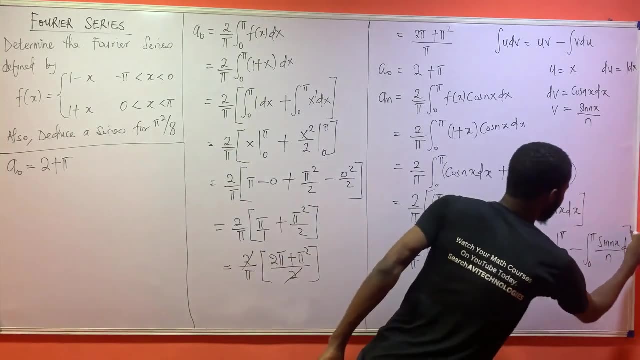 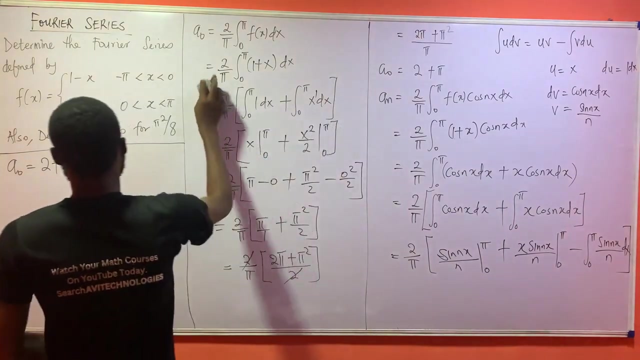 giving me dx because it said vdu and our du is equal to what one dx. so it's a very easy and simple process. let me put this guy in the bracket, let me put that very guy in a bracket. so that's what we have and i'm going to continue. i'm going to proceed at this very part. i'm going 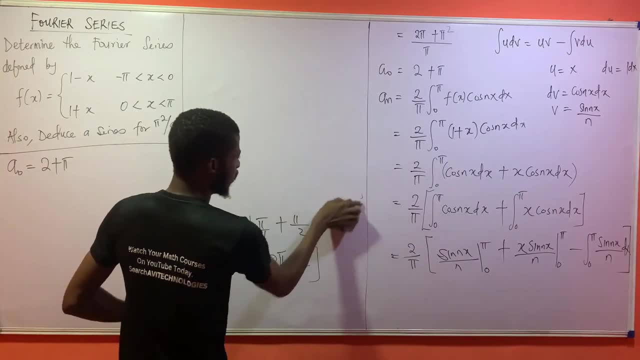 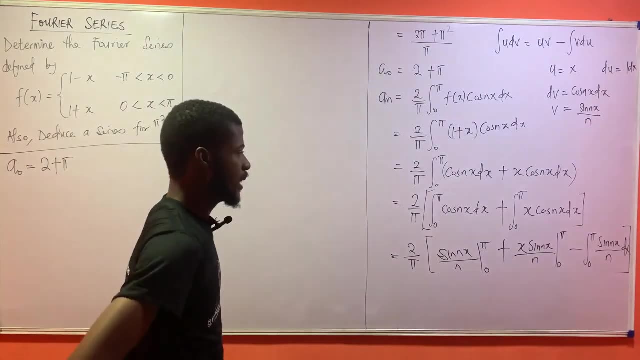 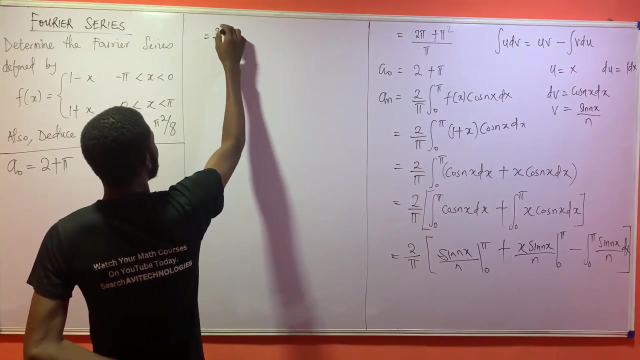 to proceed at this very part. okay, now let us look at this carefully and let us see what we can do. okay, now, look at this. let me write my two over pi first of all- so this is two over pi- then open this very bracket up now if i should take this very guy. please, please, look at this. 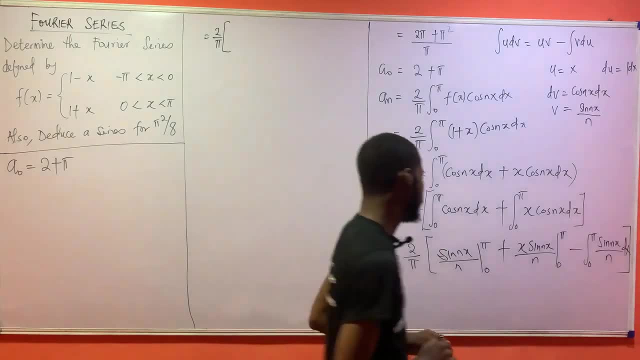 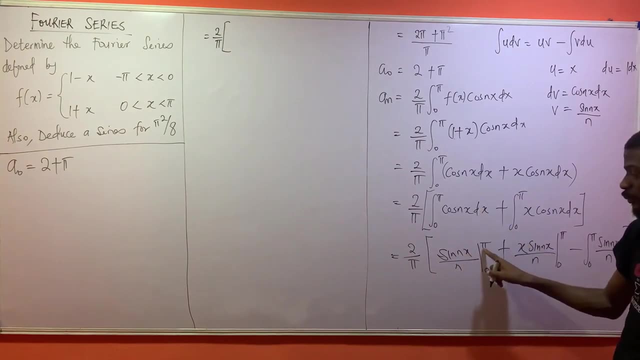 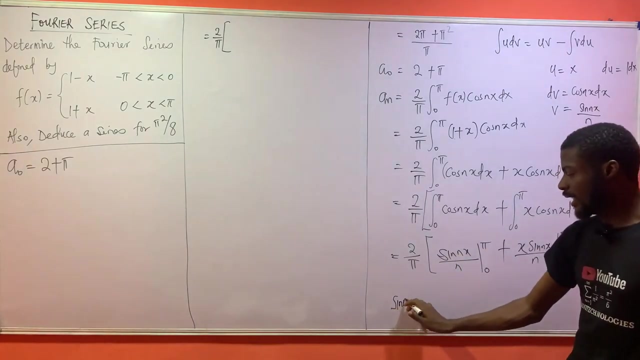 this, very everything, is going to give me zero. why did i say so? if you should put sine, you know, while actually doing everything with respect to x, right. so anyway, you see, as you put pi, sine and pi, pi is 180 degrees right. so sine and pi is always going to give you zero because sine 180. 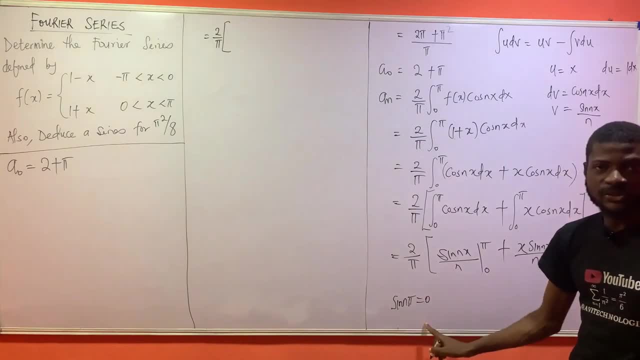 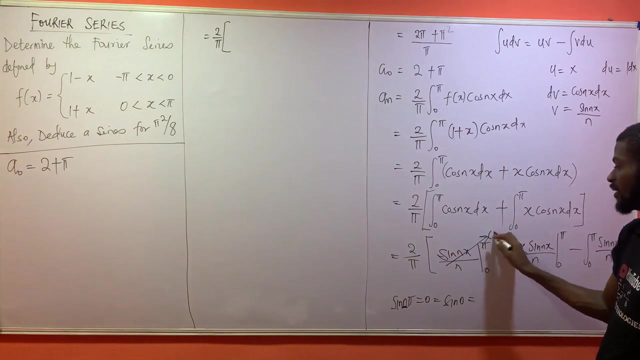 is zero. sine 360 is zero. they are all zeros. then what if you put zero as your x? sine zero is still worth zero. so it means everything here, this sine zero, whatever value of n you are going to have, your answers are going to be worth zero. so everything here is zero. everything here is zero. 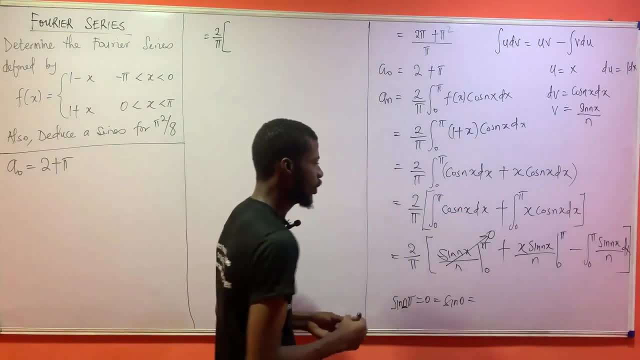 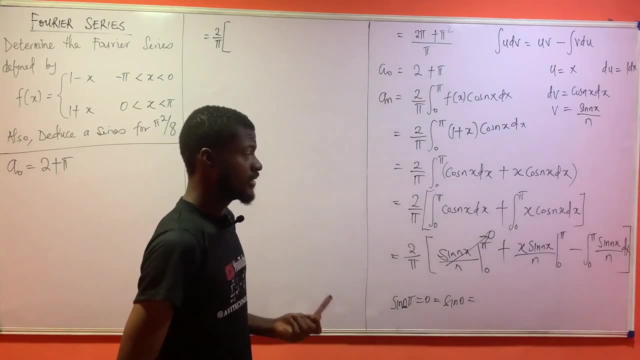 now, if you come to this part, i think yes, yes, if you come to this very part, you are still going to be getting the same thing, the same zero, the same zero, simply because, if you look at this, it's still the same sine and water view. so it's. 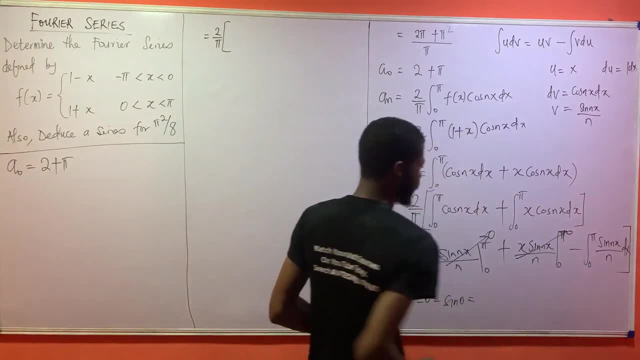 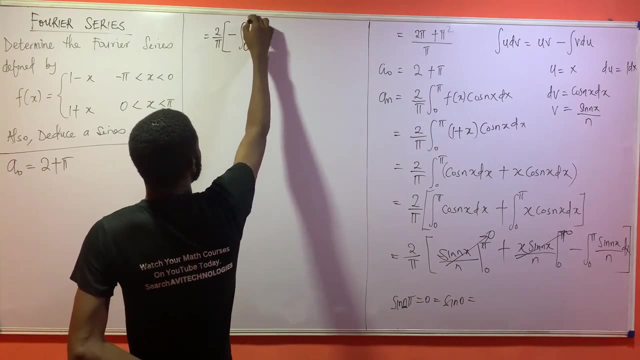 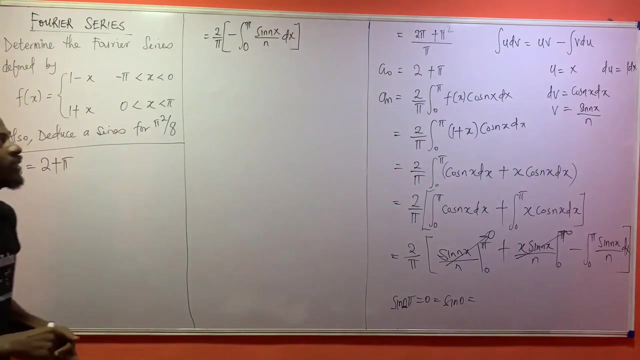 still zero. this part is still zero, this part is gone, zero. so what we'll be left? we'll be left with minus integral from um zero to pi of sine nx over m dx. okay, so this is what we have now. i'm trying to make the video as short as possible, but please you can let me know in the comments section. 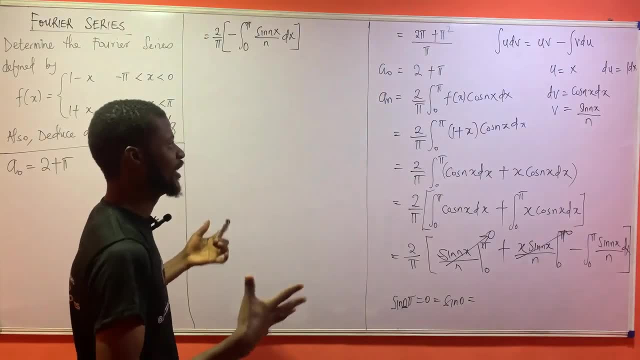 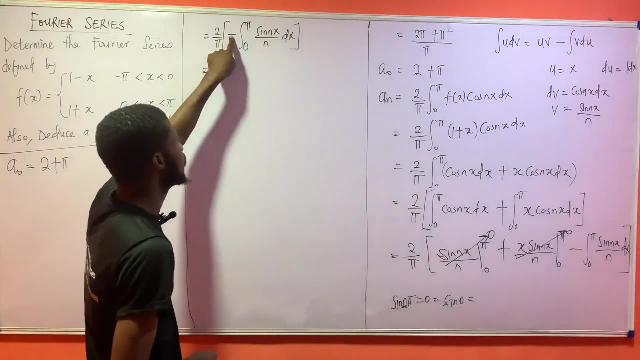 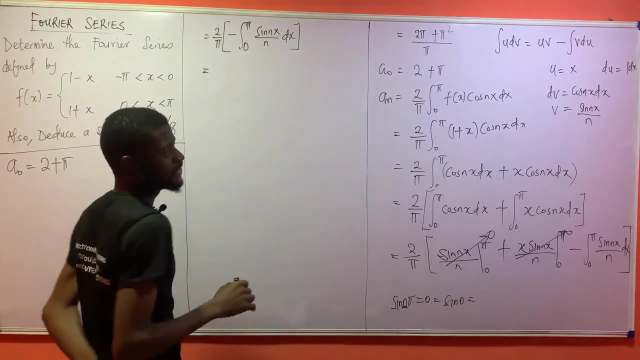 if, um, i should make it much more longer so that everything will be understood. okay, now this guy, look at this, look at this carefully. this is a minus sign, right, thank you? this is also n, since since i am actually, let's say, um different integrating with respect to x and this n is. 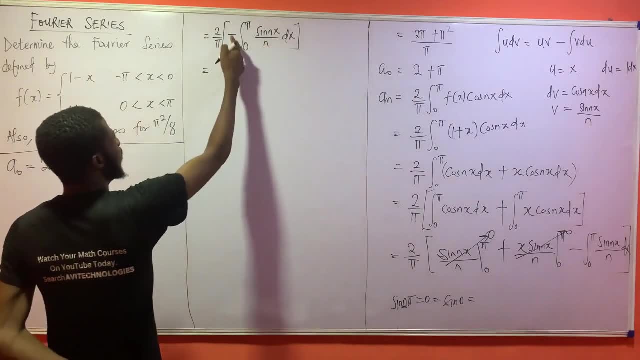 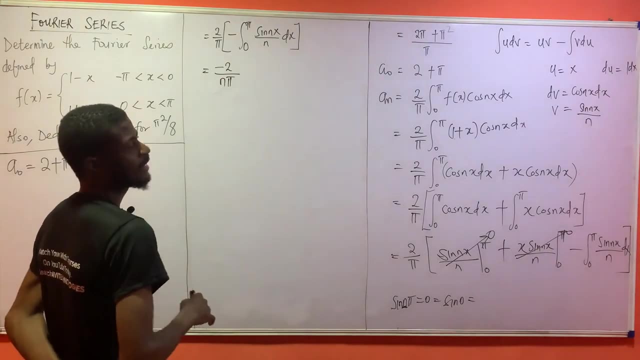 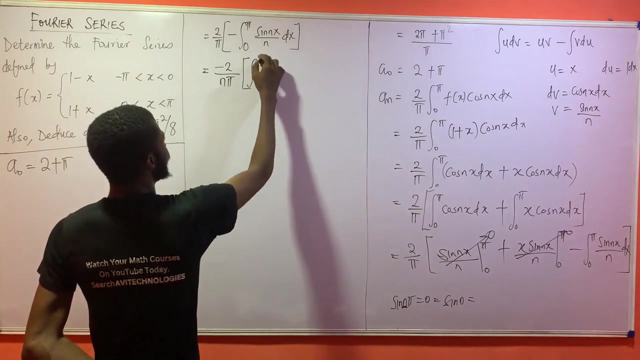 here it means n is a constant, so i can bring it out, i can bring out the minus, and so this minus 2 over this guy comes out and pi. i can do that clearly because n is a. what is a constant now, integral from 0 to pi sine n? x. 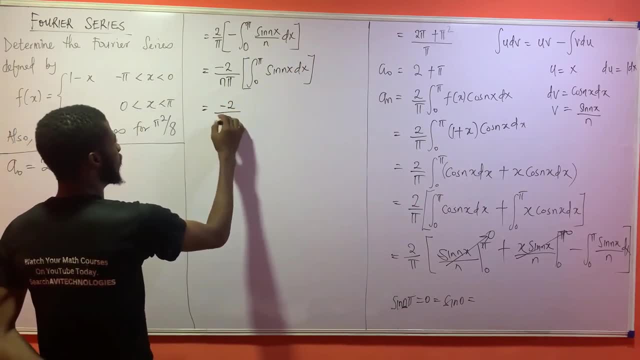 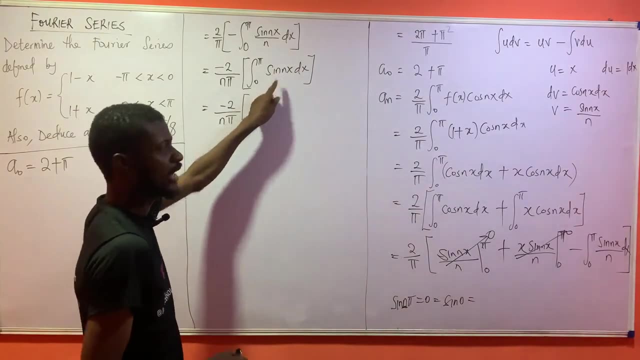 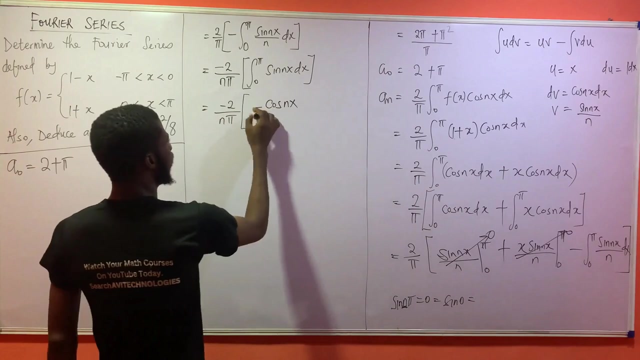 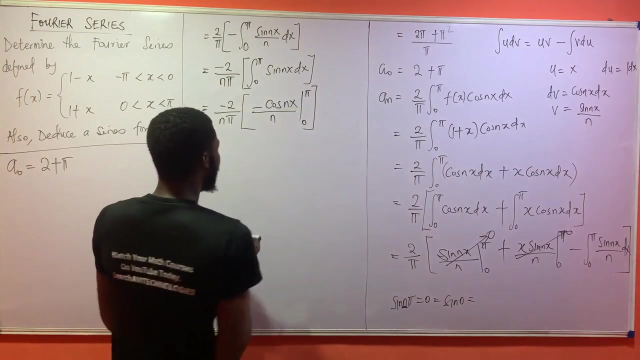 dx. okay, now this will become minus 2 over n, pi, um. how would i evaluate this? very integral. so first of all, integrate, sign. what would you get? minus cos for your start, minus cos and x, right, then, all of over, what n? then i'm going to put my limit zero towards pi. okay, so this is what i have. 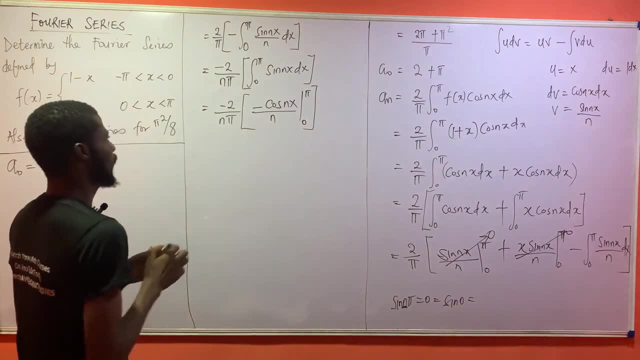 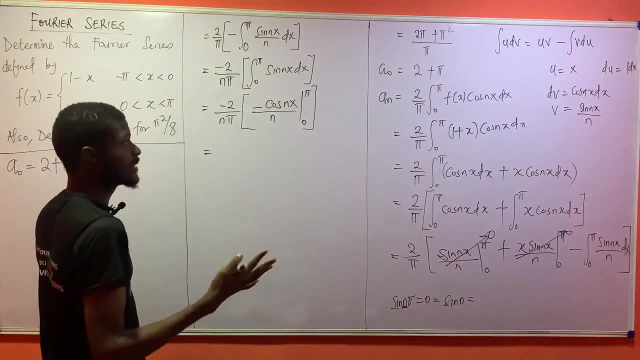 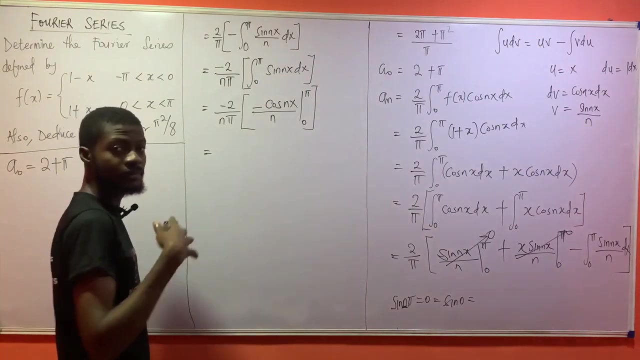 this is what we have. okay, let us continue now. looking at this again, looking at this again. minus is a constant. i can bring it out if i want to. i can bring it out then this n you see here, the n you see here, is also a constant. so if minus comes out to me, this minus i'm going to be having. 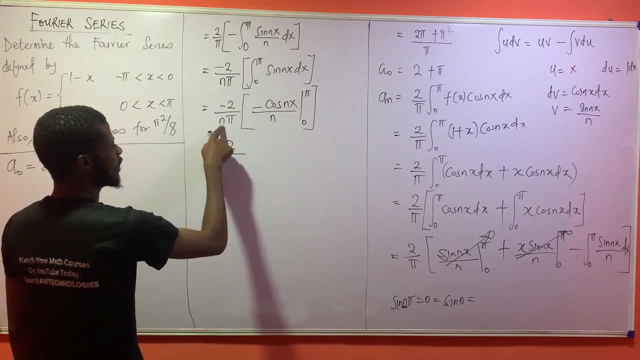 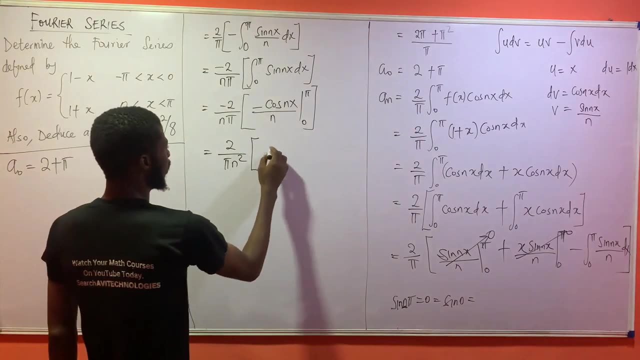 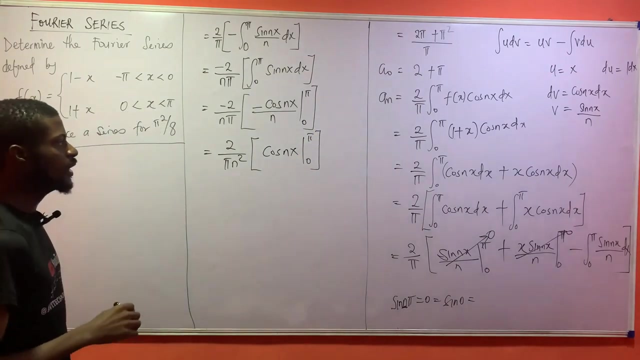 plus. so this is 2 over. if this n comes out, i'm going to be having pi n squared, because n times n is going to give me what n squared. and what do i have here? cos nx, and i have my zero towards pi. okay, now this very part. what do i do? anywhere i see anywhere, i see x. i'm going to put pi. 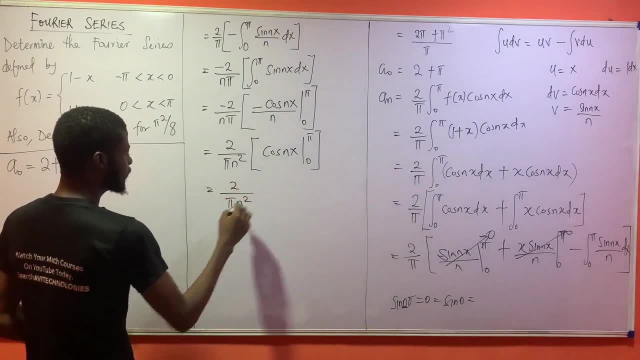 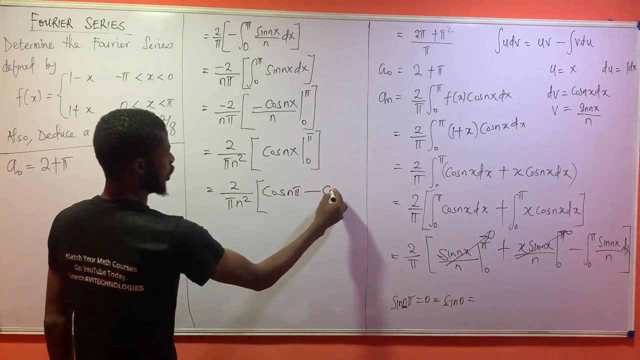 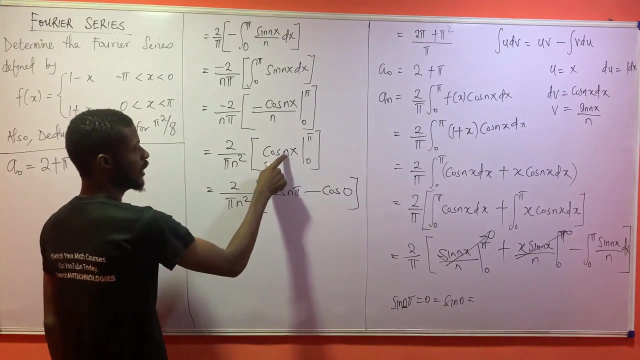 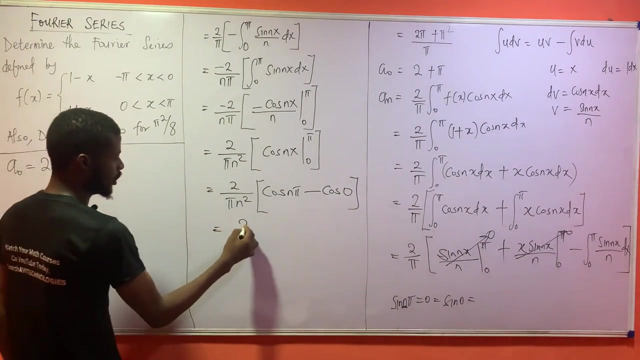 so this is 2 over pi n squared. open bracket: cos n pi minus cos zero. why, what's happening? why is it zero? simply because if i put x as zero here, n times, zero will still give me what zero? okay. so this is 2 over pi n squared, then bracket, do you? 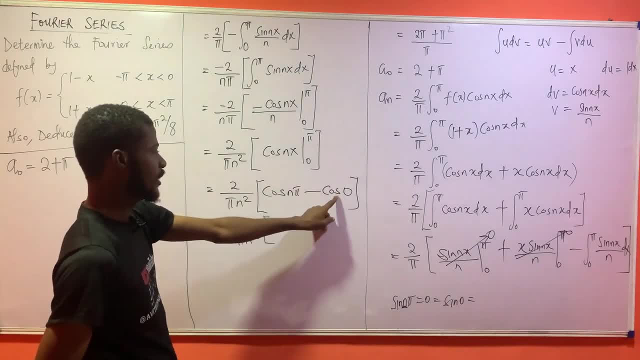 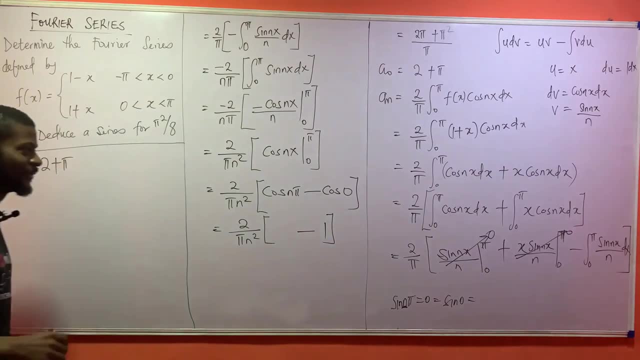 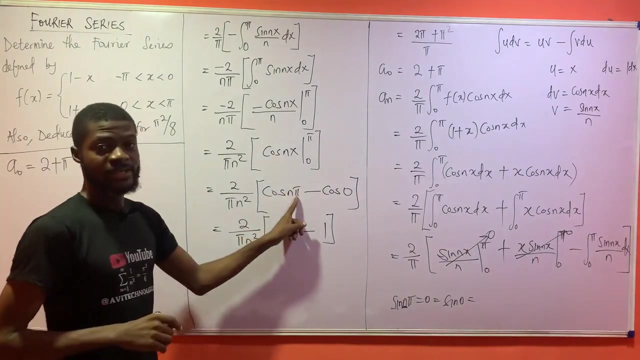 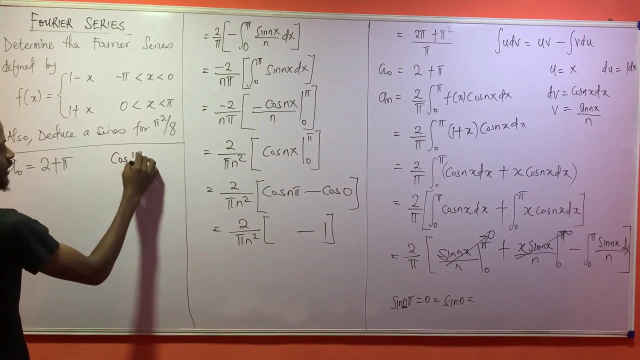 agree that this guy is going to be giving you one. this guy's going to be giving you one because cos 1, so this is minus one. i don't really know what's happening. okay, now, cos n pi. now, please take note of this. pi is 180 degrees, right, thank you. pi is equal to 180 degrees. now, see, come here. cos 180 degrees. 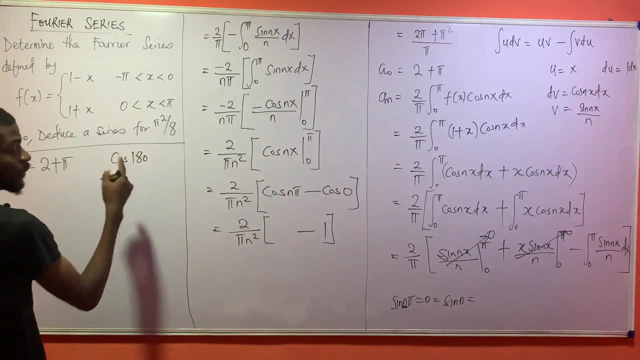 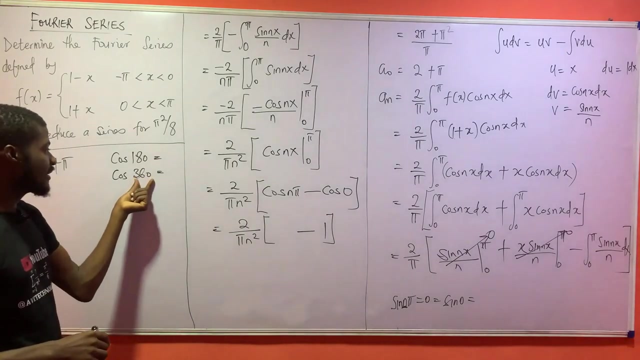 please take note of this. cos 180 degrees- we're going to be assuming so many things. cos 180 degrees, it's going to give you a particular answer. cos 360 degrees, it's going to give you a particular answer. now please look at this. if this is: cos 360 degrees, cause 360 degrees, cause 360 degrees. this. 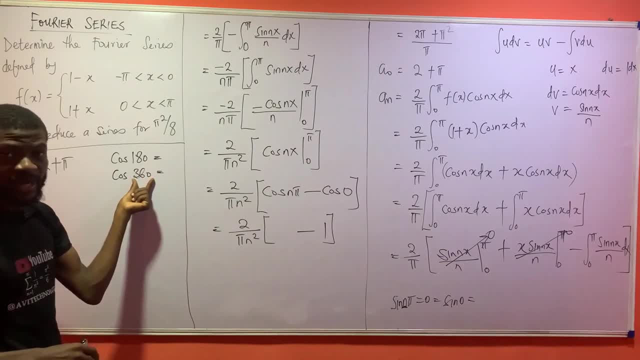 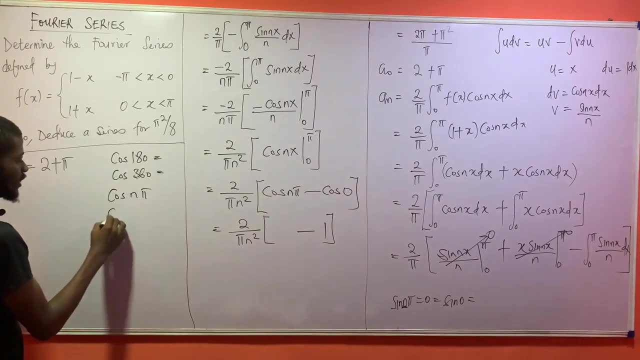 is even right, because, see, we have cos n pi. let me explain this properly. we have cost n pi. now this is cos n can be any number can be 1, 2, 3, 4, 5, 6, so but just know, we have 180 degrees times n. now, if n is, 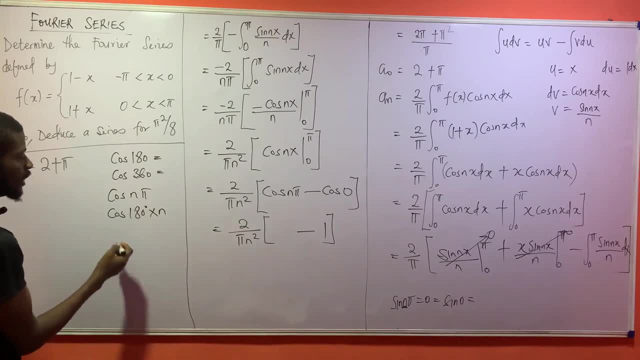 1, which is odd. your answer here is going to become 1, so you would notice that in pi this is no. yeah, so this is equal to n times n, because this ch Nina rule is that only one is a enter. that rule is equal to x. so we get this and we will need to write this down. of course, there are even degrees times. why? because if we get the same answer that i'm not going to get, so it will be: say what we got, so now, where is the answer here? so the answer here is going to become what? because x is the right answer. this is going to be a kind of a. 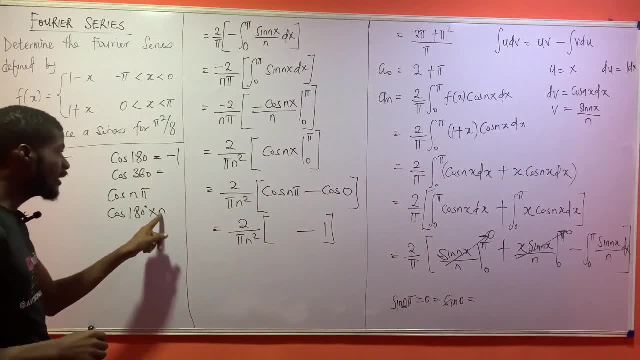 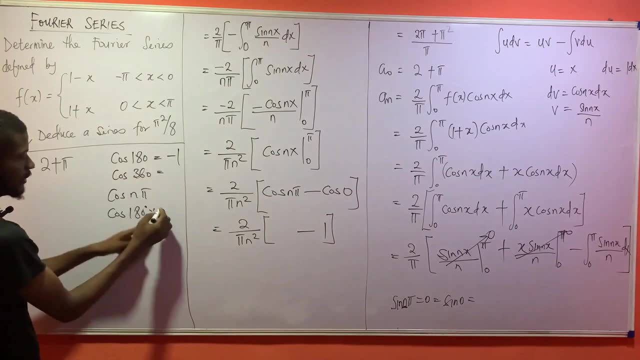 going to become what minus 1. if n is odd, your answer is going to become what minus 1. now, if n is even this 360 case, let me say n is 2, for example, 2 times 180 will give you 360. so this: 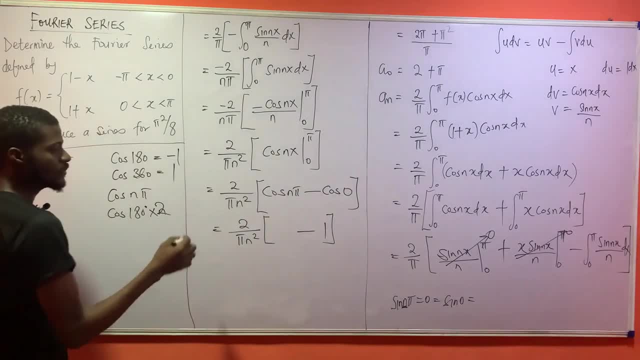 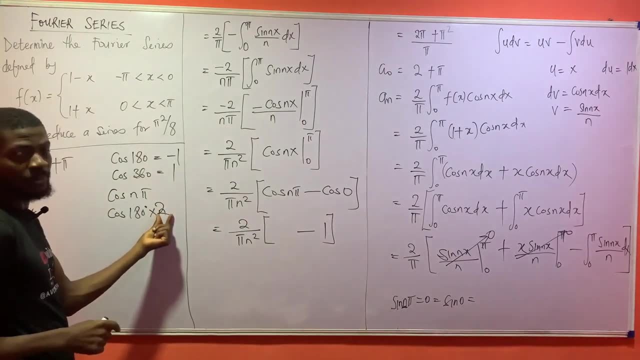 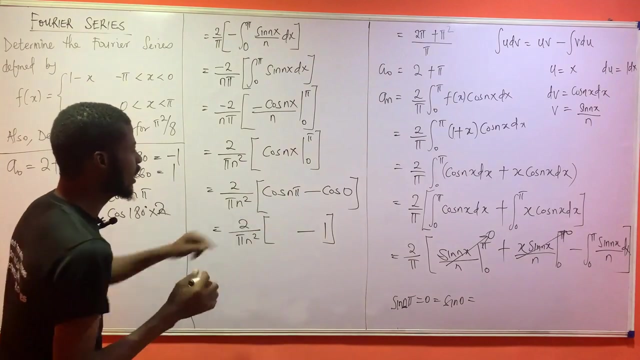 will give me what? 1 now, what we didn't notice here. this guy. this guy, if i have even, i'm going to be getting plus 1 because i tried it with an even number. it's giving me plus 1 because the values of cos n pi rotate between 1 and minus 1. some textbooks might even come here and write minus 1. 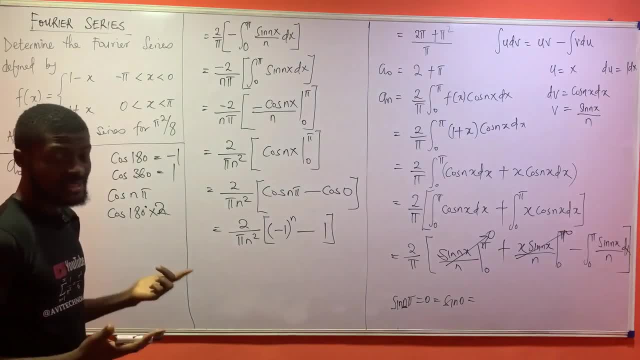 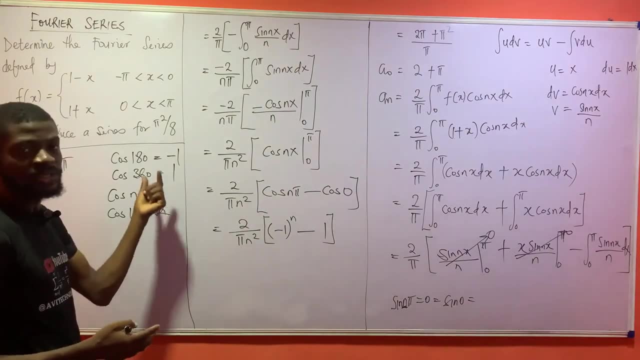 to the power of what n some textbooks might do that, so they are still going to be correct, because the value of this guy alternates between 1 and minus 1, depending on if it's odd or what. even if it is odd, you're going to get minus 1. if it is even, you're going to get 1. now, so let me just 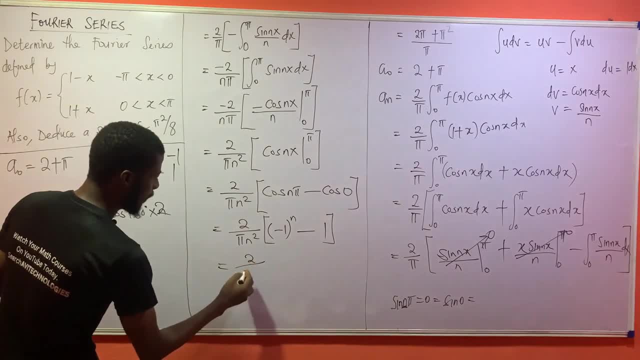 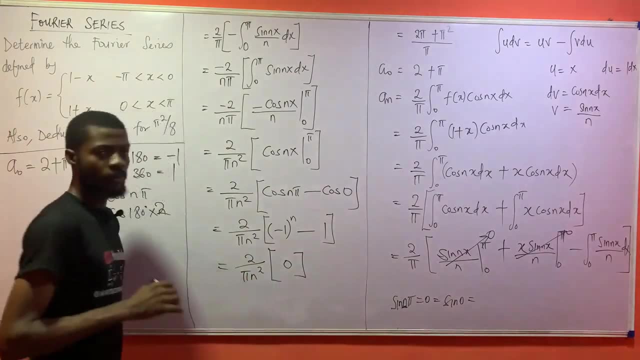 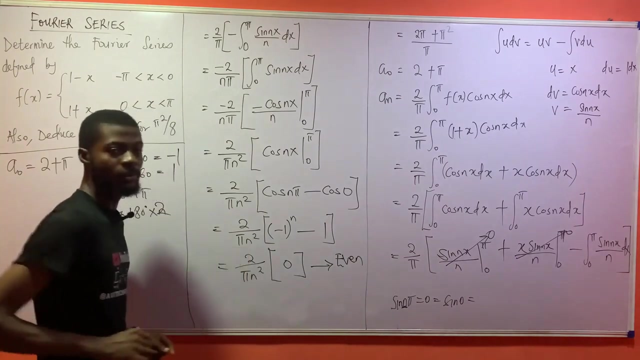 leave it like that. now, this is 2 over pi n squared bracket 0. now why do i want to pick 0? i don't want to pick 0. if it is even, i'm going to put this answer here. if it is even, this is going to become my answer, because if it is even my answer, 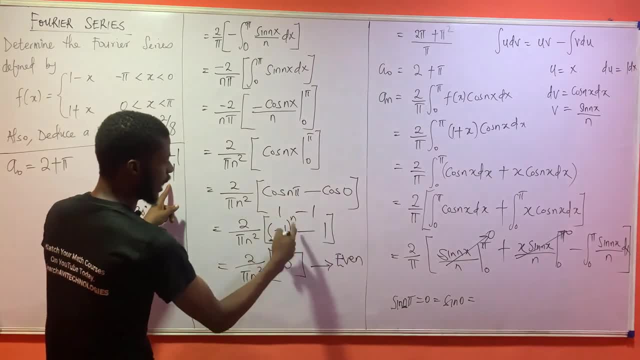 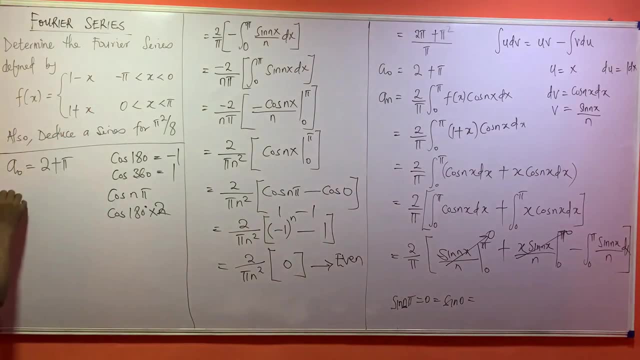 is always 1. so if you say 1 minus 1, your answer is going to be 0 and anything times 0 is going to be giving you what 0? so it means a. where is this guy? a sub n is equal to 0, when we have even. 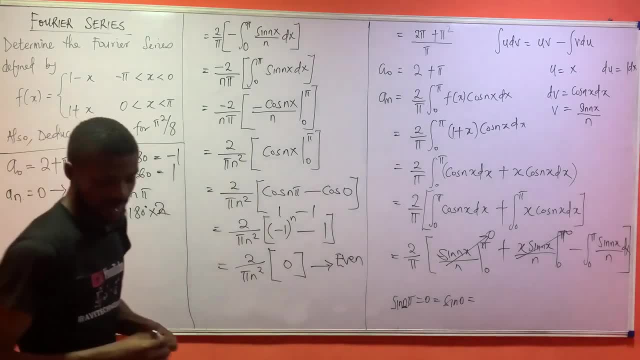 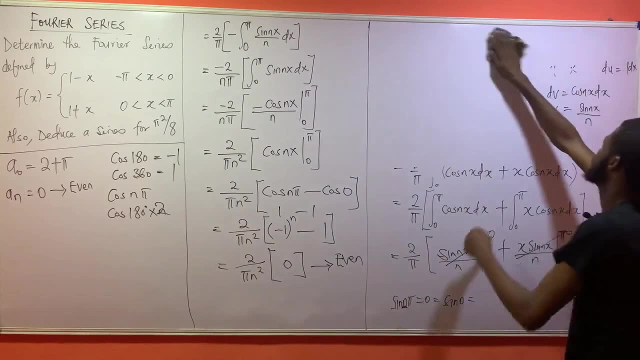 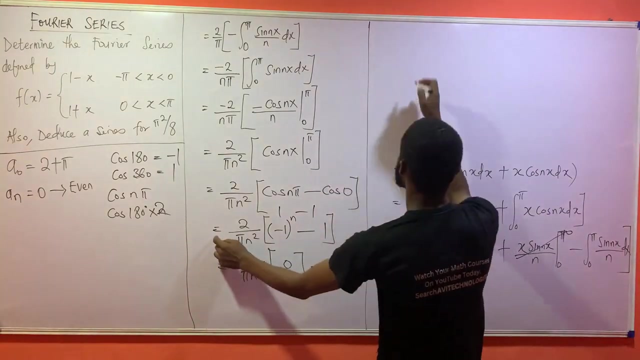 values for n. now, what if we have odd values for n? what if we then have odd values for n? what would happen if we have odd values for n? what would then happen? now, see, i'm going to be saying, uh, where's this guy? this is what i have. so i have 2 over pi n squared bracket minus 1 to. 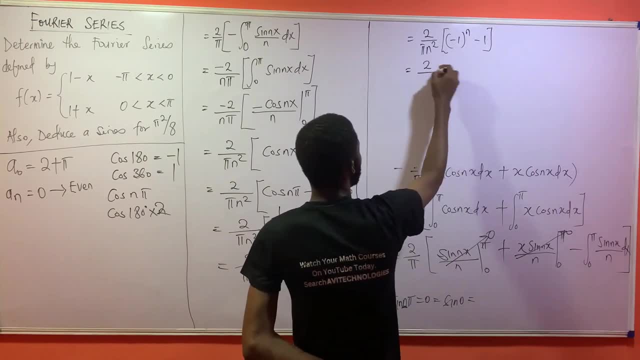 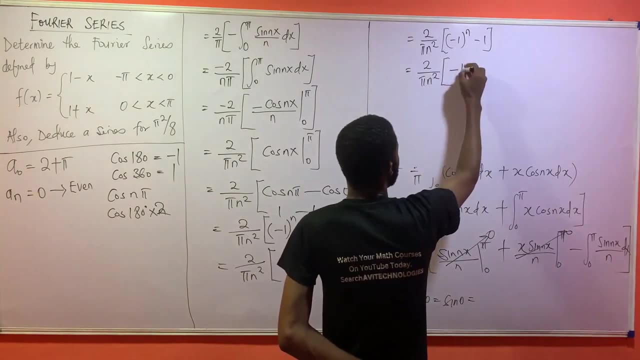 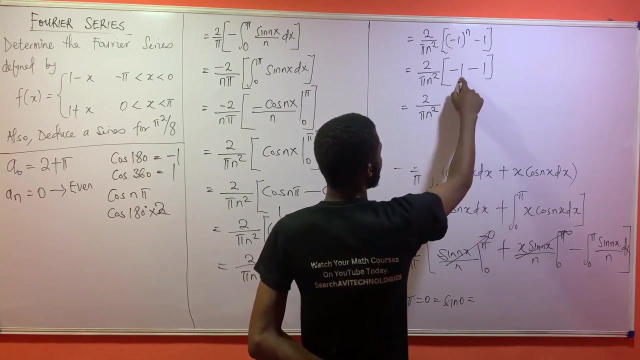 the power of n minus 1. okay, now this is 2 over pi n squared. imagine if this was odd now. if this is odd, it means i'm going to be having minus 1 minus 1. if it is odd now, this is going to become 2 over pi n squared. minus 1 minus 1 is minus 2. this is going. 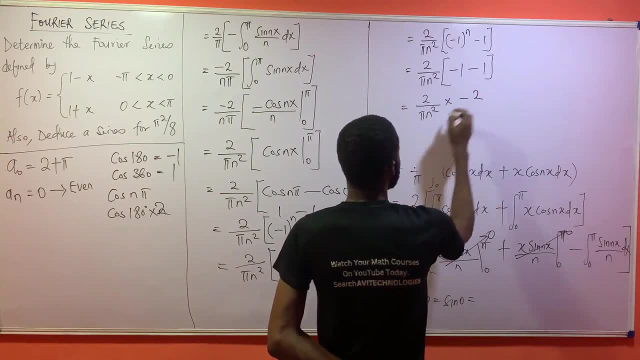 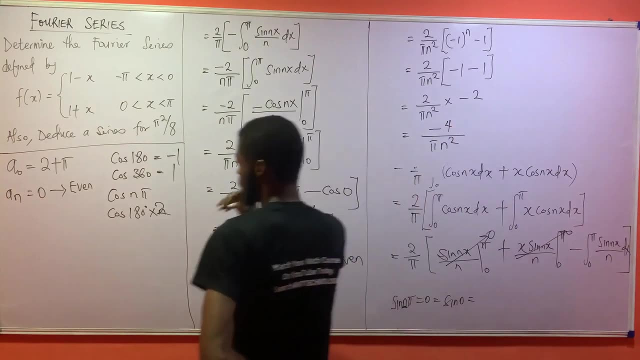 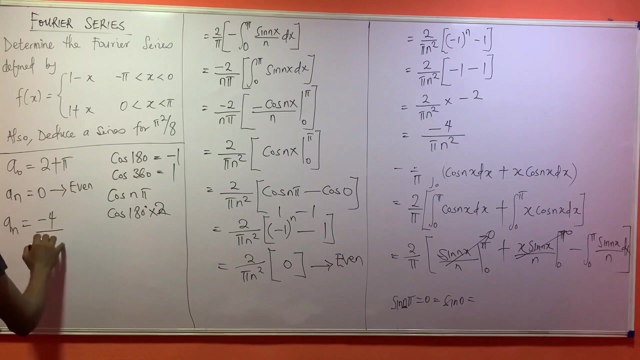 to be giving me minus 2 this times minus 2. now this will be giving to me 2 times minus 2. is what minus 4 all over what pi n squared? so it means a sub n is equal to um minus 4 over pi n. okay, let me write the pi first: pi n squared. so this is what i have for that. 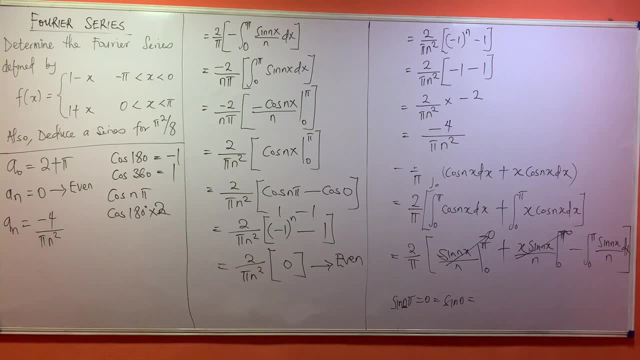 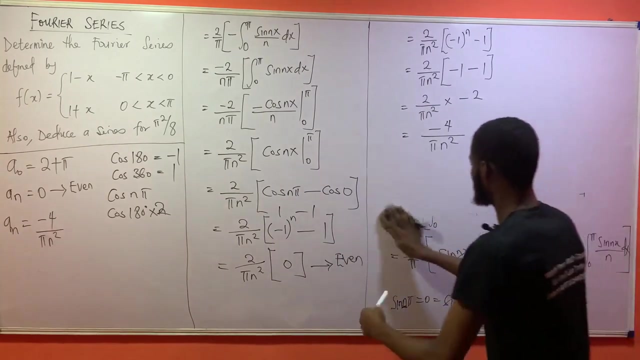 that is what i have for that very guy. so if i'm done with all of this, the next thing i'll then do is to evaluate what i have, is to evaluate what we have. okay, where am i going to work? okay, this very side. so those values are very, very 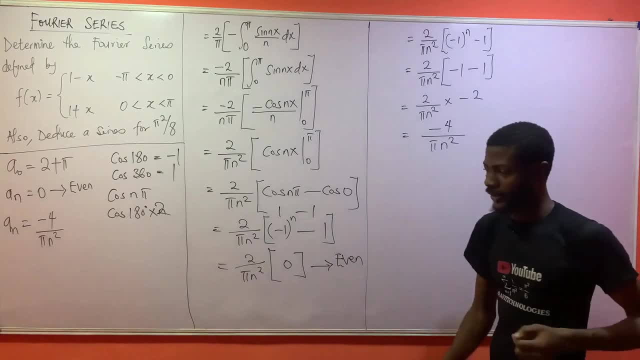 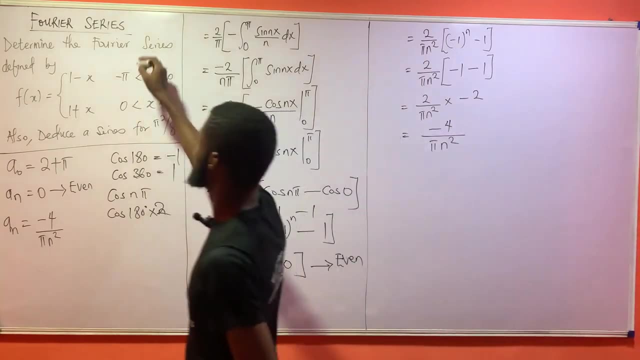 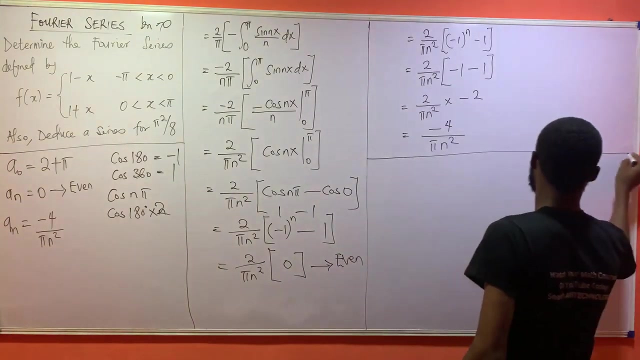 correct. those values are very, very correct. okay, now did i find b sub n? no, remember, if this guy is an even function, b sub n is going to be giving you what zero. it's going to be giving you zero. so let us continue here and let us see what this will give to us now for even functions f of s. 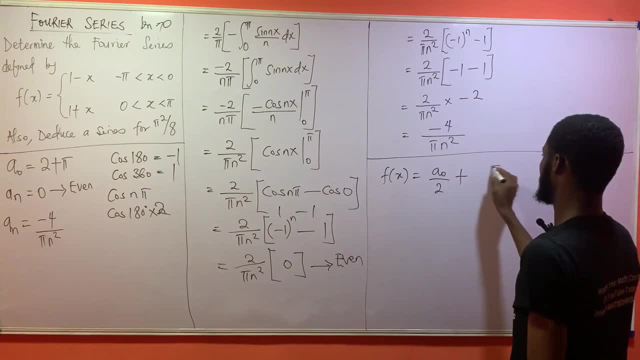 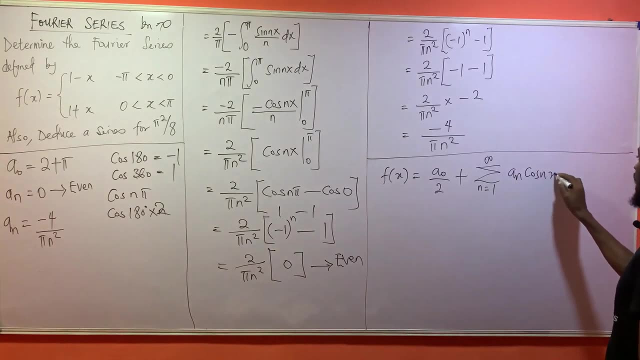 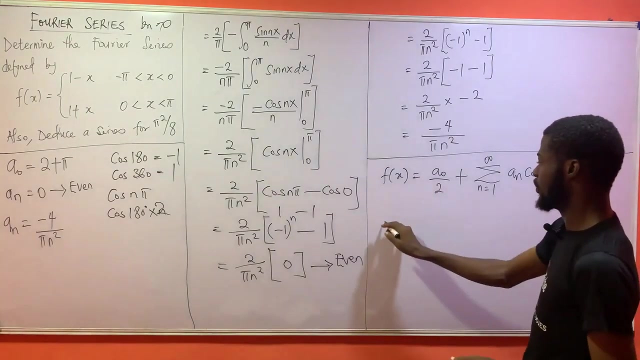 is equal to a naught over 2, plus the summation from n equal to 1 to infinity, of a sub n cos nx. now the reason why i did not write b is because it's going to be zero. this is an even function. now this is going to become f of s equal a naught. what is a naught? a naught is: 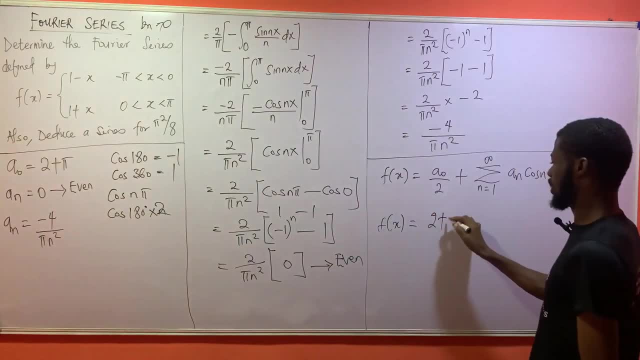 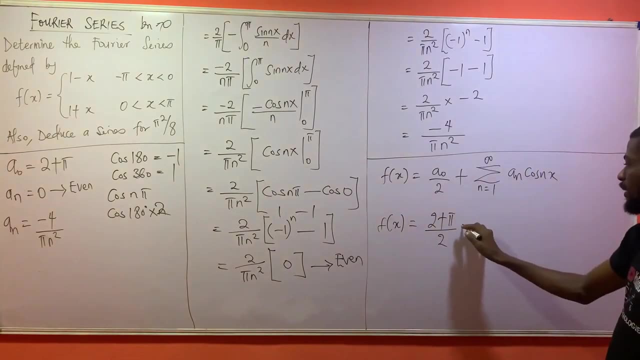 2 plus pi. i'm going to say 2 plus pi over um 2, so this will have 2 plus pi over 2, then plus the summation from n equal to 1 to infinity of 2 plus pi over 2. so this is going to become f of s. 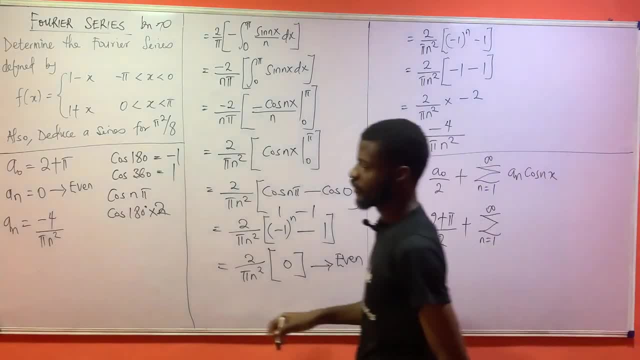 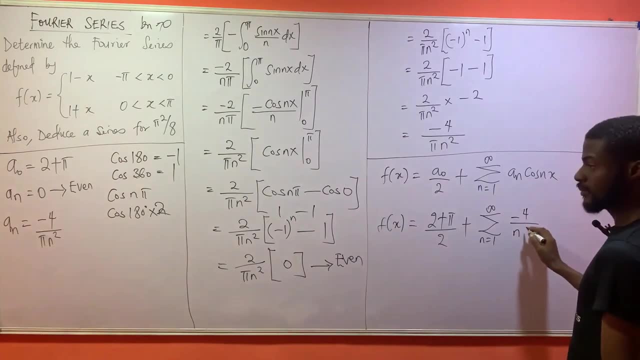 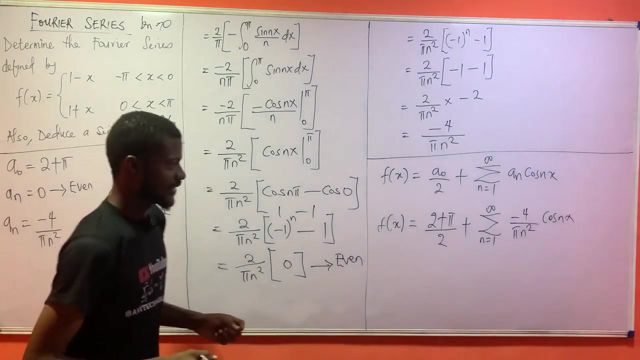 equal to 1 to infinity. a sub n is what minus 4 over, what minus 4 over n? okay, i don't know, i write writing my n first, pi n squared, okay, then cos nx. so this is what i have. okay, i'm just trying to be strong for this, just trying to be strong. okay, i'll go see my. 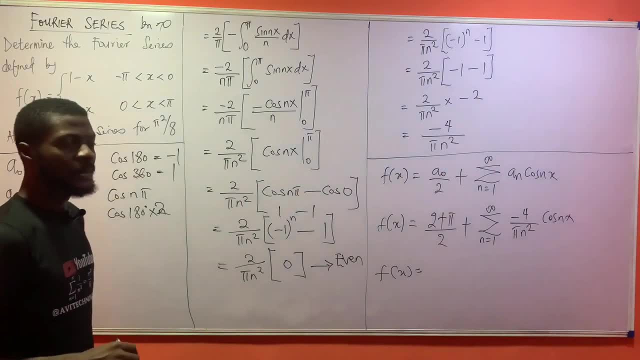 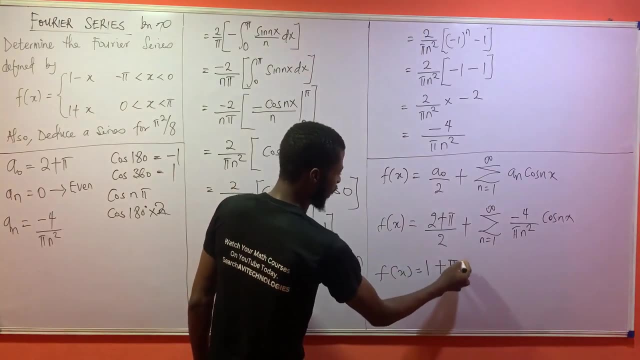 doctor very soon. okay, now let us see what will be the next thing i'll do. can i actually say 2 over 2, 1 then plus pi over 2? you know i can do that right? yes, it's possible. i can do that. it's very, very possible. now look at: 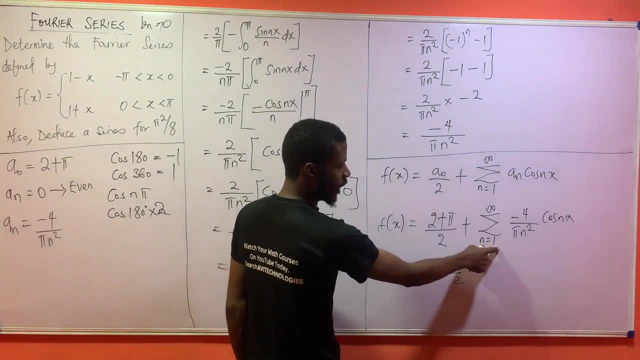 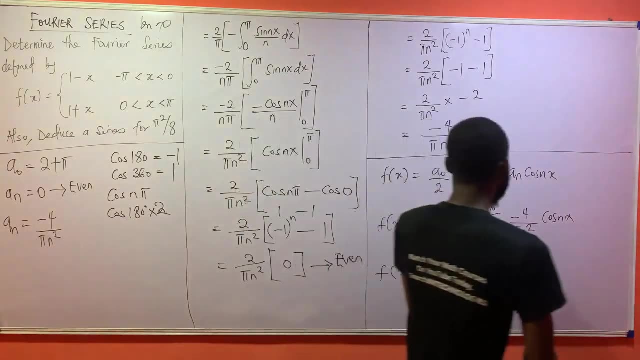 this: the variable here is n equal to 1, right, so it means any other thing that does not have n is a constant, it can come outside. so it means this minus 4. you are seeing this minus 4. you are seeing. and this pi. you are seeing that constant is a constant. so it means this minus 4, you are seeing. 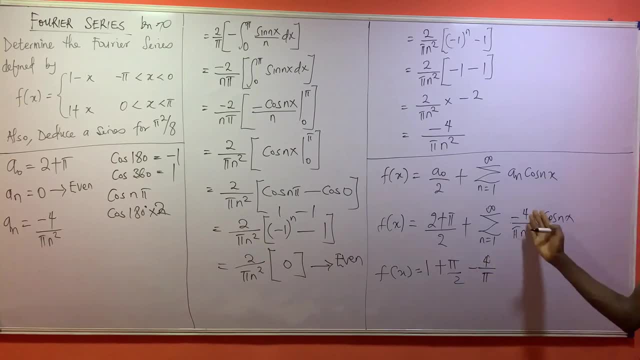 a constant, this minus 4 over pi. because they are constant, they can come outside from n equal to 1, to infinity of what will be remaining here: 1 over n squared of cos nx. now, remember what am i going to be picking? i'm going to be picking only the odd terms, because if it is, 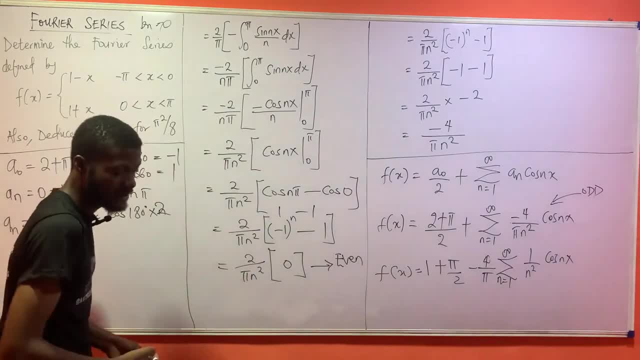 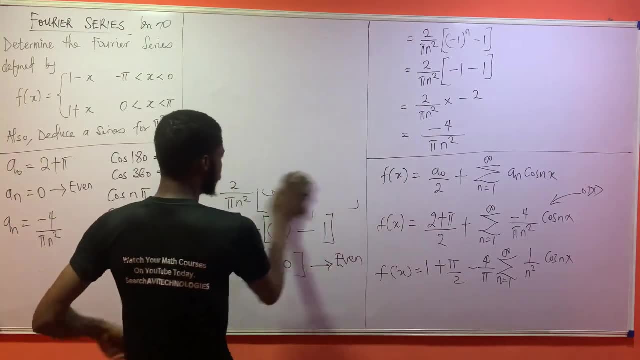 even you're going to get zero, this, even you're going to be getting zero, okay, well, i'm almost through with this, almost through with this. so i'm going to be getting 0, because i'm going to be getting 0 with that. i'm almost through with it. okay, so this is going to be giving me f of s. 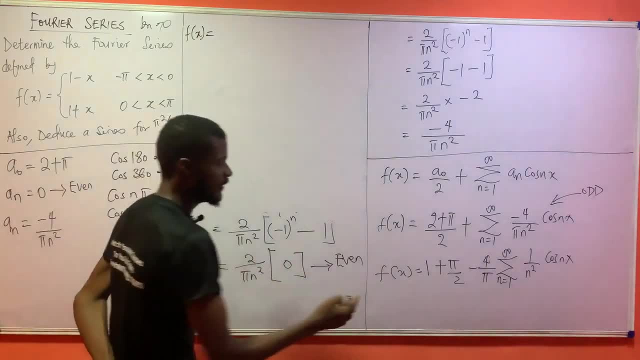 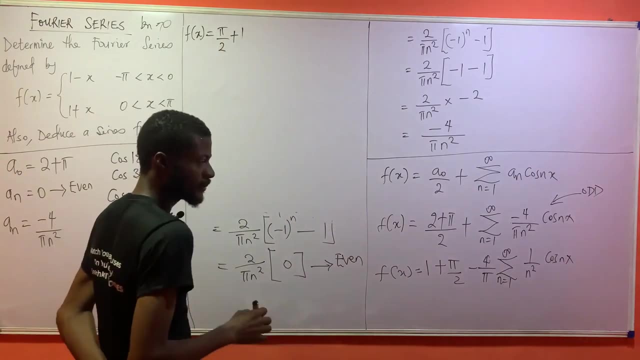 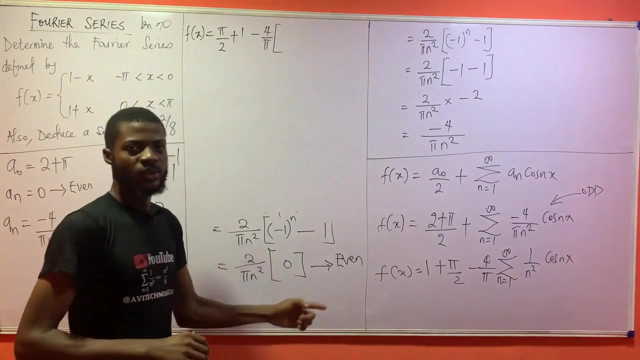 equal. is it better if i write pi over 2 first of all? i can do that. i can write pi over 2 first of all. then plus 1 minus 4 over pi. open a bracket now. let us start evaluating this and let us what the values are going to become. let us evaluate and see what the values are going to become. 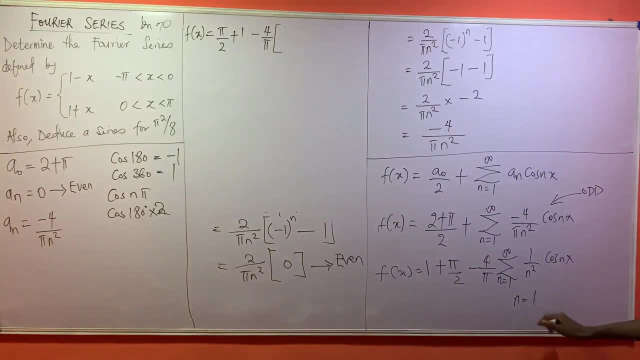 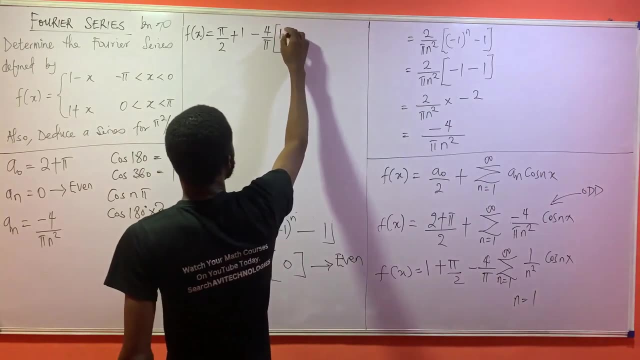 now, for example, if i write pi over 2 first of all, i can do that. i can write pi over 2 first of all for n equal to 1, n equal to 1, 1 squared is what 1. so 1 over 1 is still 1. so i'm going to say 1 cos s. 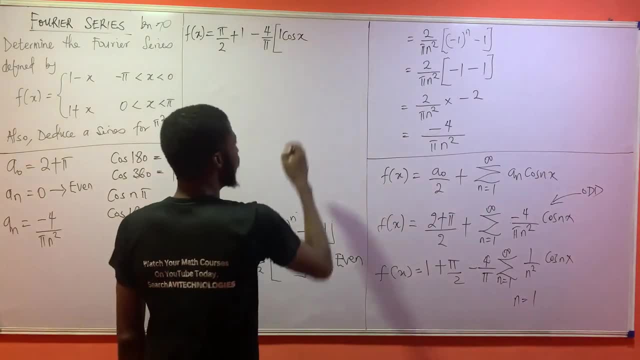 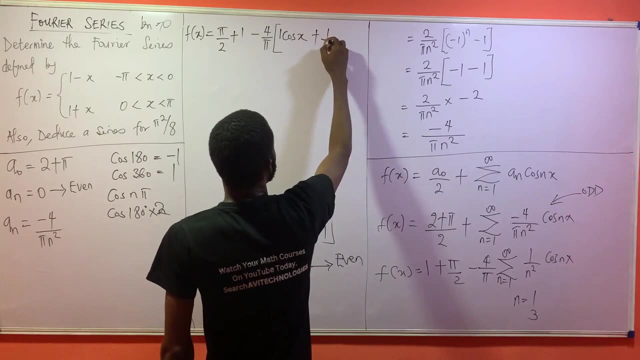 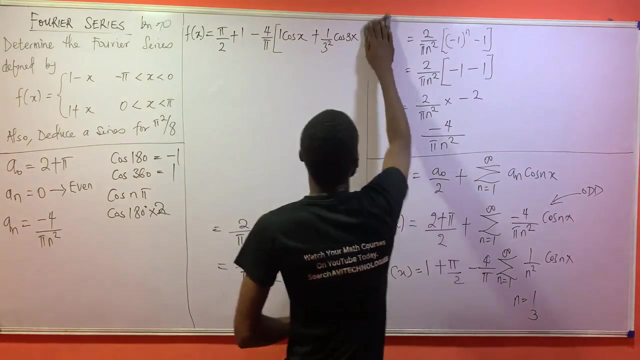 it's not really a must for you to put the 1 in front plus what is the next odd term, 3. so i'll say 1 over 3 squared. 1 over 3 squared, cos what the next one is going to become what it's going to become. 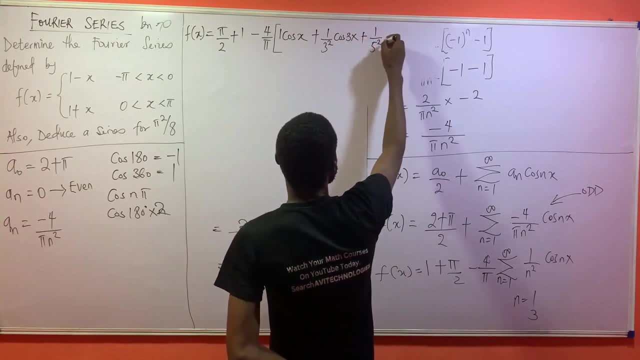 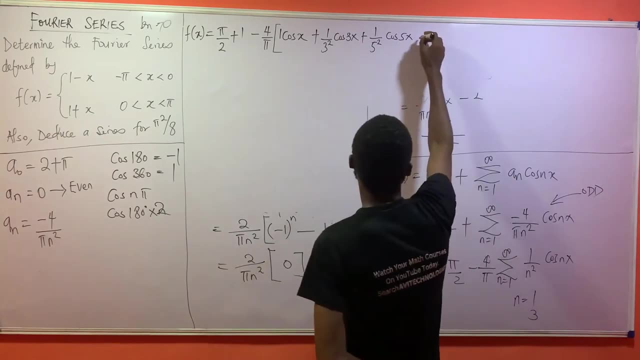 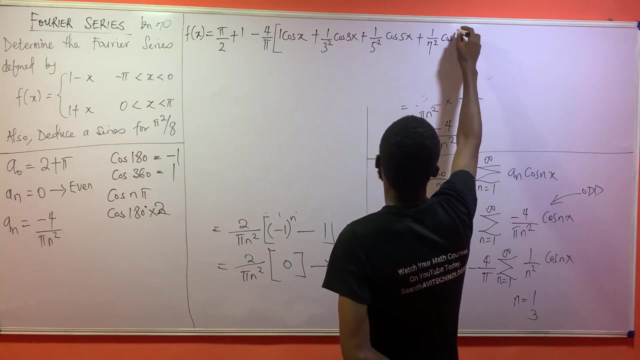 plus 1 over 5 squared cos. what 5s? because anywhere i see n, i'm replacing it with what? a another number after 5, the next one is 7. so this 1 over 7 squared cos 7x, then plus. it goes on. 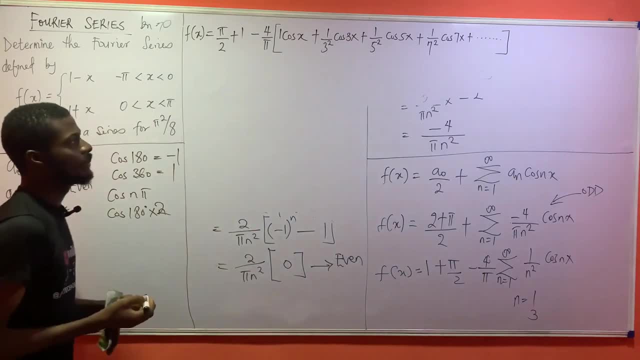 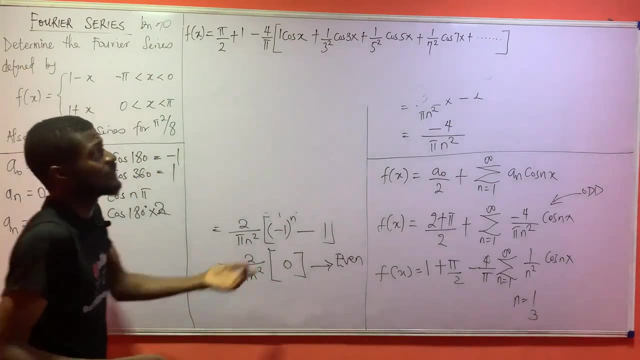 like that. it continues. so this guy can be called the fourier series. so if they say determine the fourier series, this is your answer. so this guy can be called the fourier series. so if they say determine the fourier series, this is your answer. many times you can never end here. then you put: 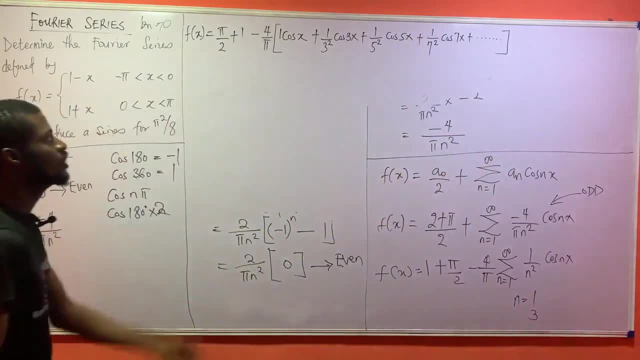 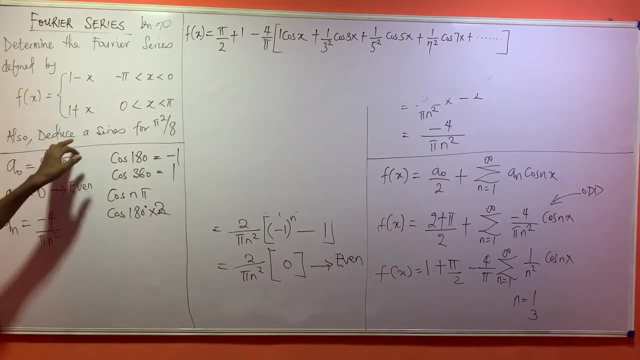 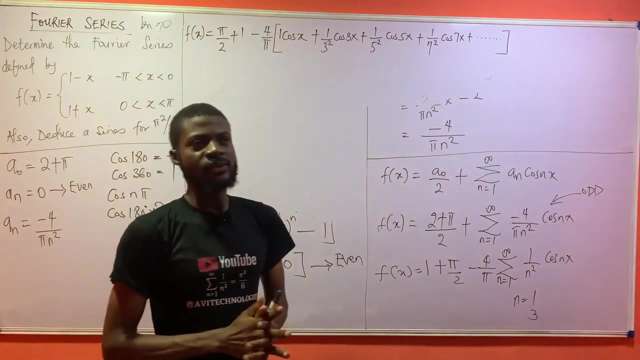 many times, you can never end here. then you put your your infinite dots. you can do that. so this guy is the fourier series for this very function. now the next question says: deduce a series for pi squared over eight. now, look at this. there's actually a theorem which i did not want to use yet. 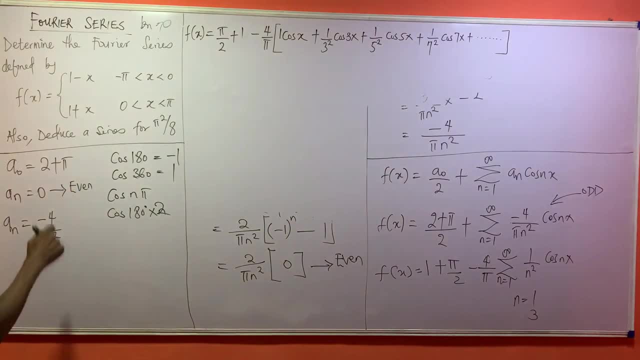 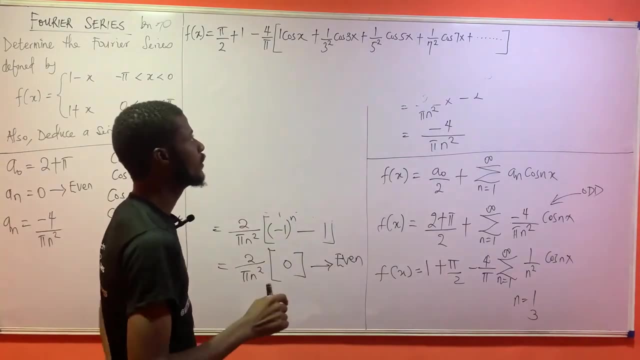 but see, there's actually a theorem but i don't wanna use it. it deduced a series for pi squared. deduced a series for pi squared over eight. now, is it possible that in one way or the other? is it possible in one way or the other that i 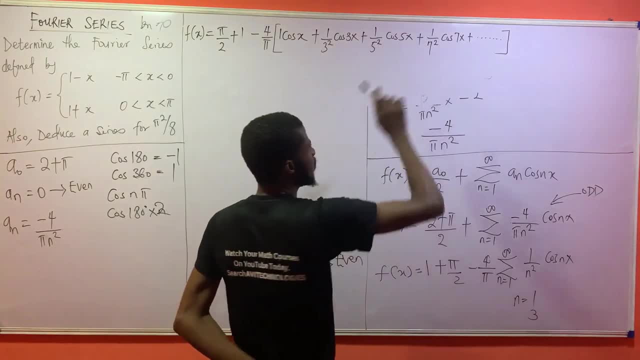 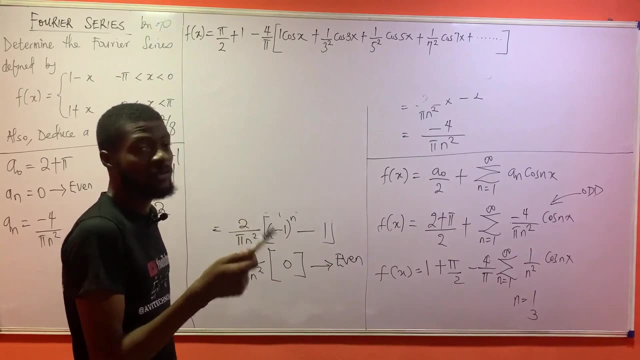 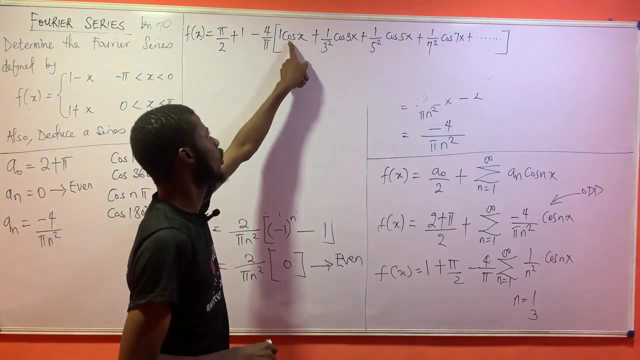 remove all of these cosine terms. is it possible? because i need a series. i can remove the cosine terms many times. it might even tell you that, oh, let the value of s be so, so, so. so now here, if i should put s as a particular value, will you notice that? because s will just disappear and will not. 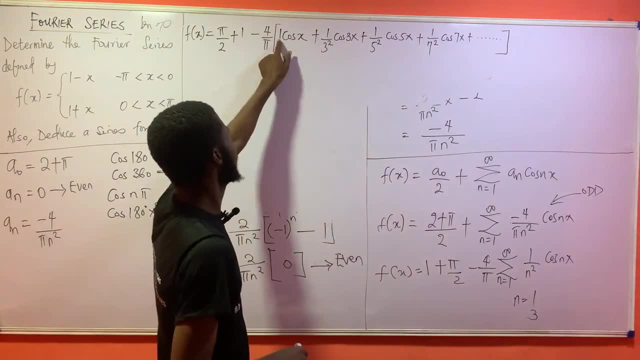 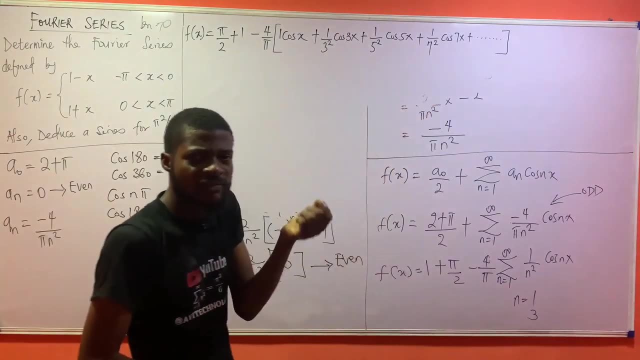 really affect all of these products. one is going to times cos x, this guy is going to times cos x, this will times cos 5x and so on and so forth. it's the particular value of s they are going to pick and it won't affect the modification. remember that anything times one is what that same thing. 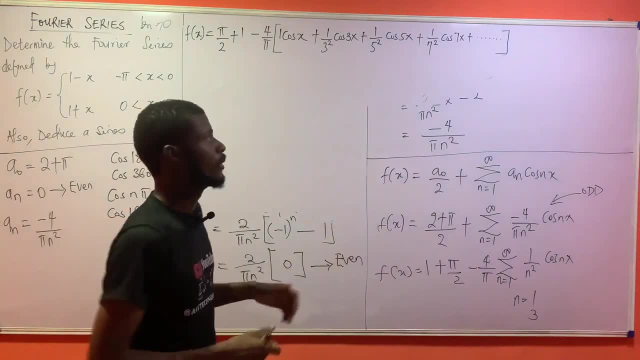 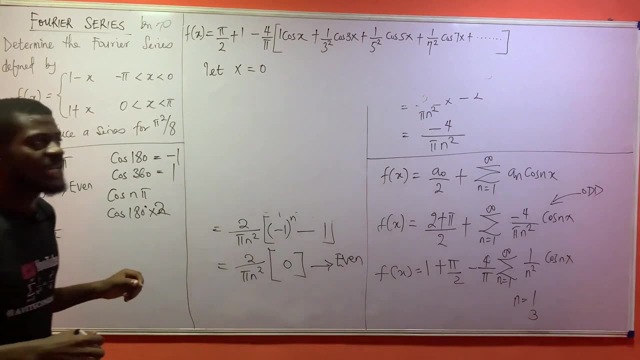 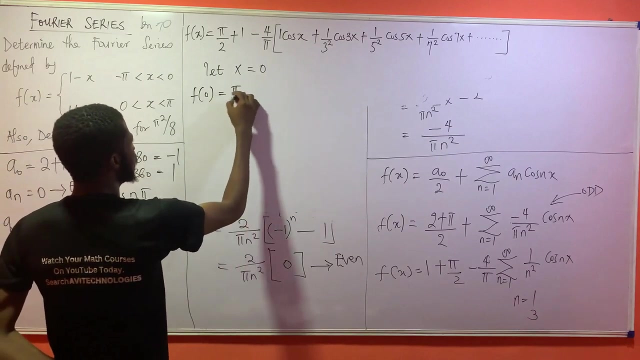 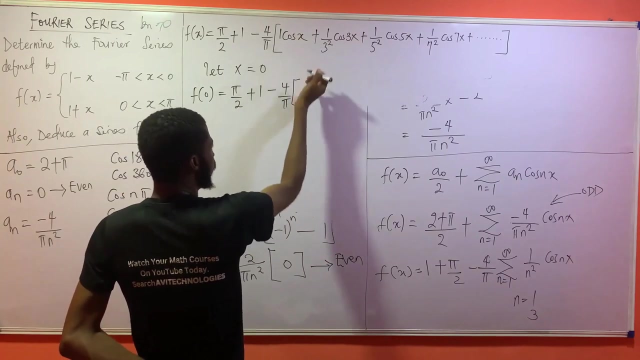 and cos what? we give you one zero. so i will say, let s be equal to what zero? so i'm doing the b part now. so let s be equal to zero, and this will become f of zero, f of zero. equal pi over two plus one minus four over pi of um, this guy is cos zero, which is one. 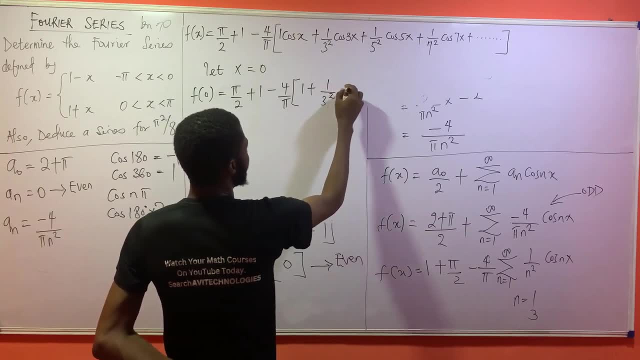 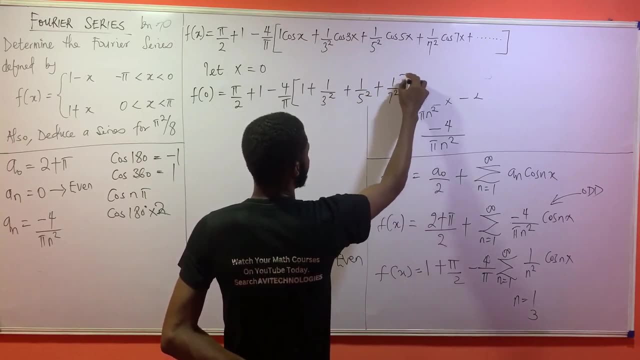 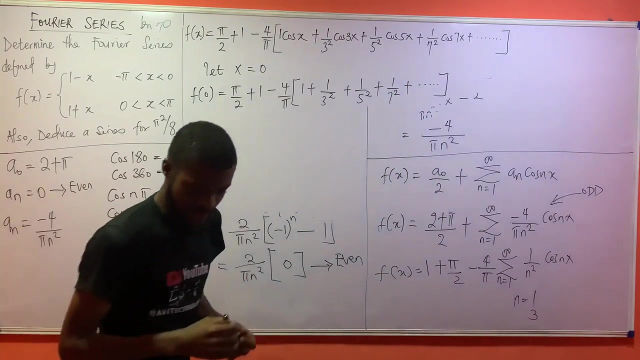 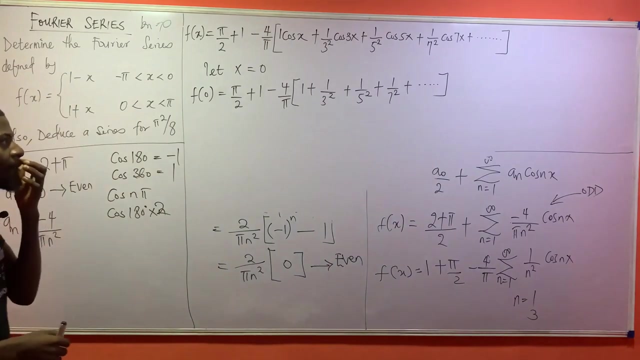 plus one over three squared, because this is now zero, which is one plus one over five squared plus one over seven squared. sorry, okay, plus okay. let me close this up like that. so this is what we have. this is what we have. okay. now, if you look at this carefully, what is f of zero? 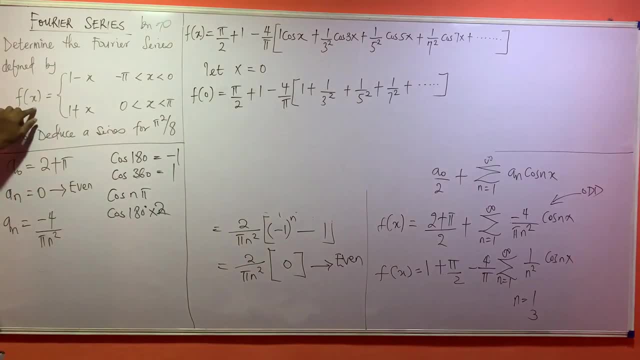 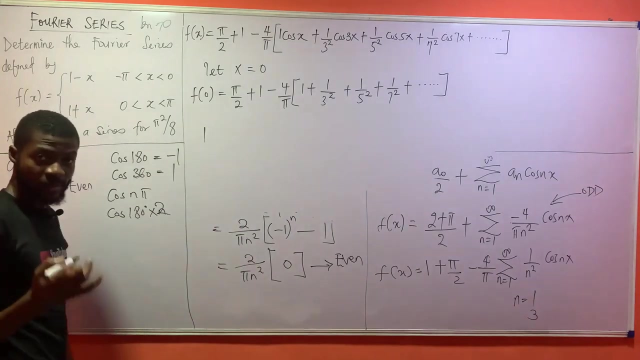 what is f naught if it is f of x and i put zero here? one minus zero is what one? one plus zero is what one? it simply means that the value for f naught will give me one, because on both sides actually one, so i can remove this very place and i put one. i believe you agree with me. so this is. 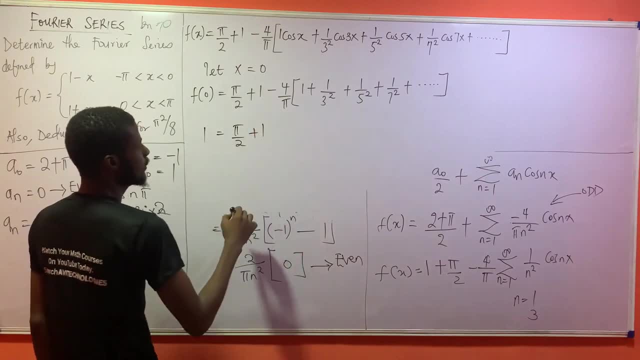 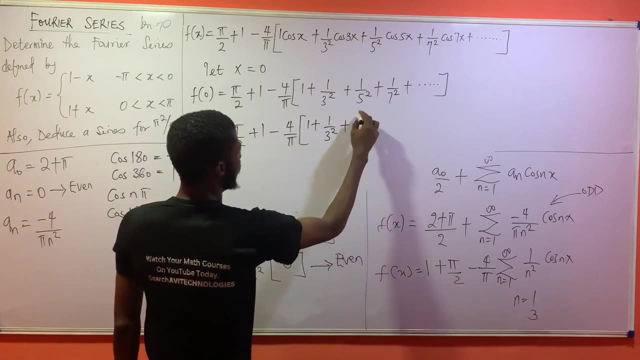 one equal pi over three squared. so this is one equal pi over three squared. so this is one equal pi over two, plus one minus four over pi open bracket. one plus one over three squared, plus one over five squared, plus one over what seven squared. then plus continues that way, okay. 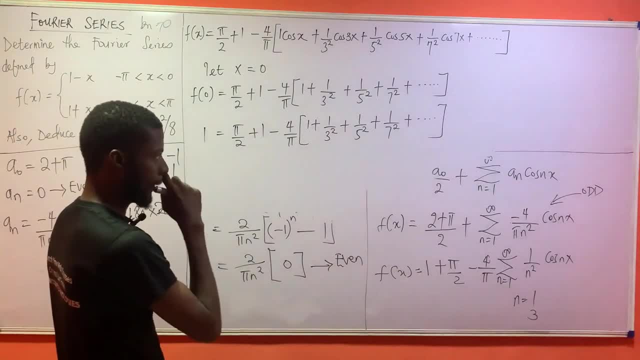 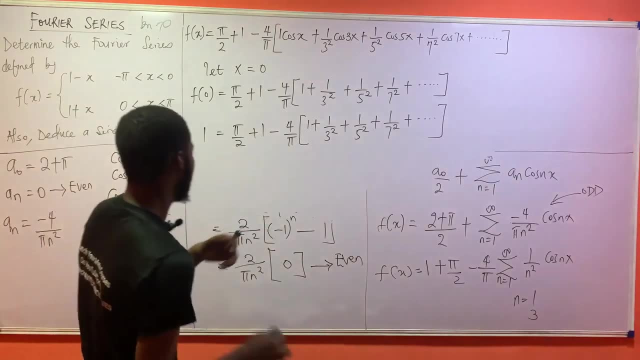 now, what will be the next thing i will do at this very part? what will be the next thing i'm going to do now? to start with, i think, let me just wipe out every other thing continuously, so i'll have the whole space to do that. so i'm going to do that. so i'm going to do that. so i'm going to do that. 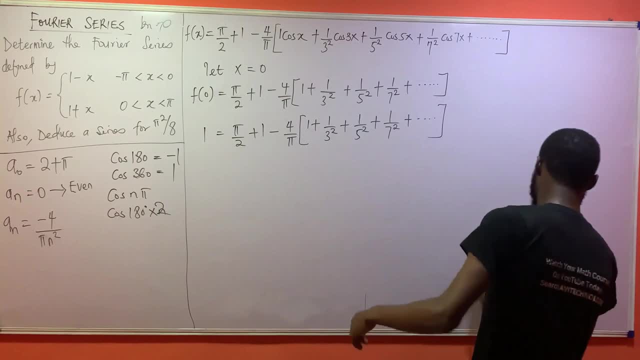 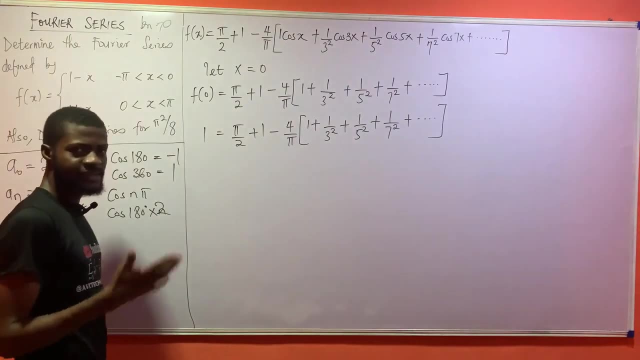 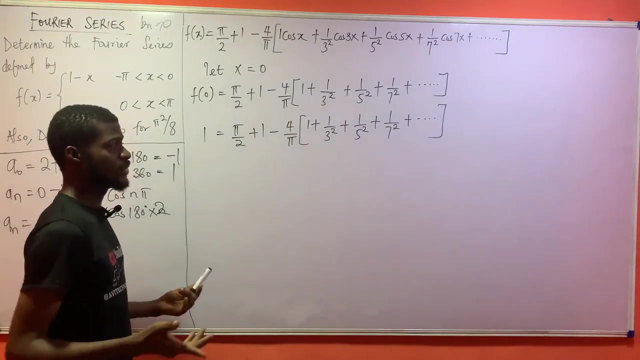 to myself, remember, i'm trying to make this video as short as possible. okay, now over the next thing i'm going to do here. can i say in one word the other that this is one right, this is also plus one. you can actually go, they can just cancel themselves. but let me not do that yet before. 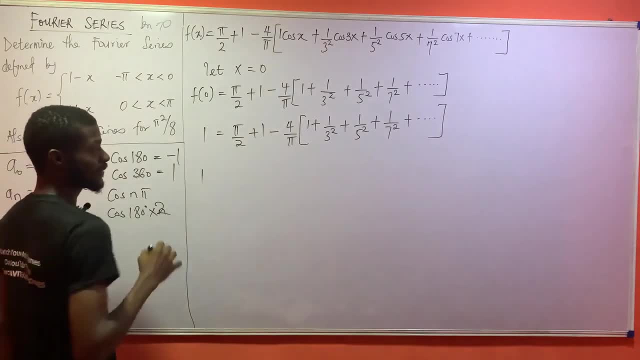 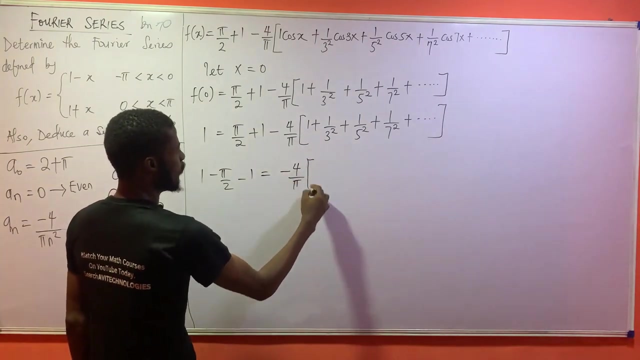 you. you will not like it. now, this is one right. you agree with that. if this pi over two can already become minus pi over two, i believe you agree with that. plus one comes up, comes minus one equal to what will be left on this other side. minus four over pi. of what? one plus one over three squared, plus one over five squared. 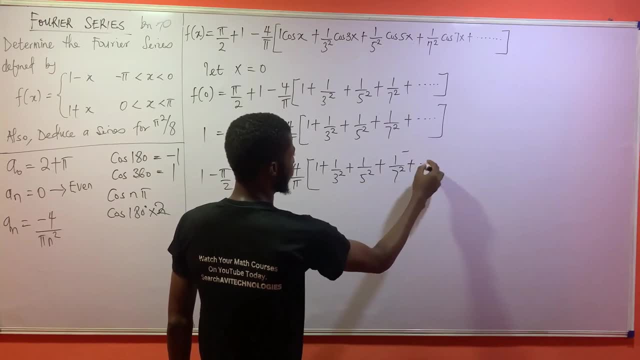 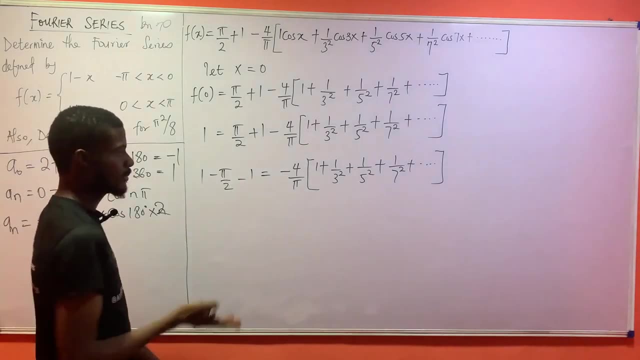 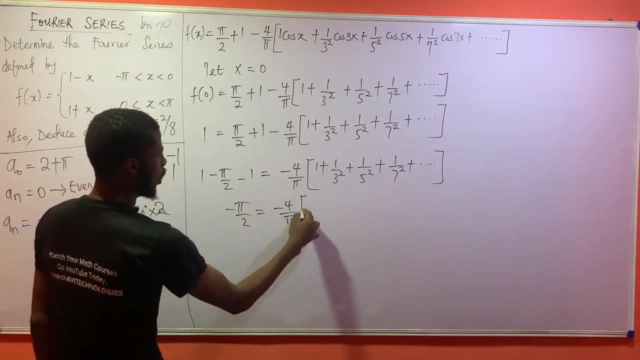 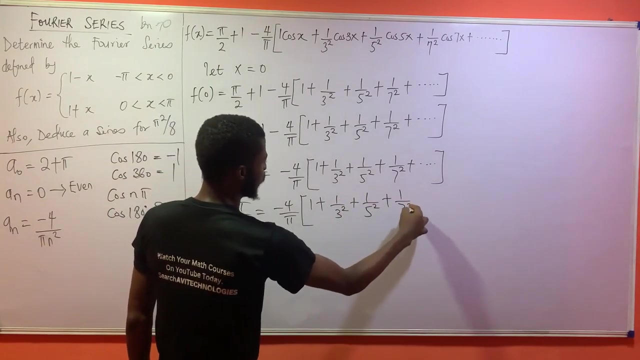 plus one over seven squared, then plus okay. okay, now let's continue. one minus one is gone, right, so that's gone. what will be left here? minus pi over two, equal minus four over pi of what? one plus one over three squared. plus one over five squared. plus one over seven squared. 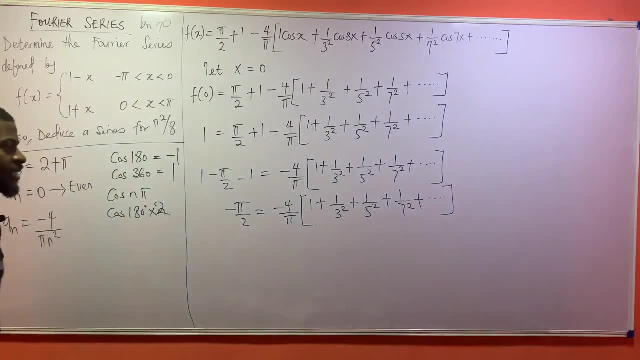 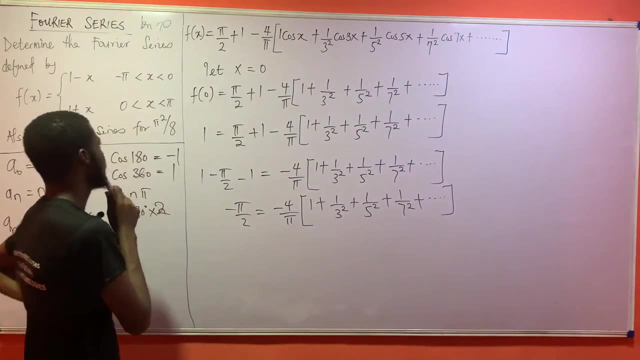 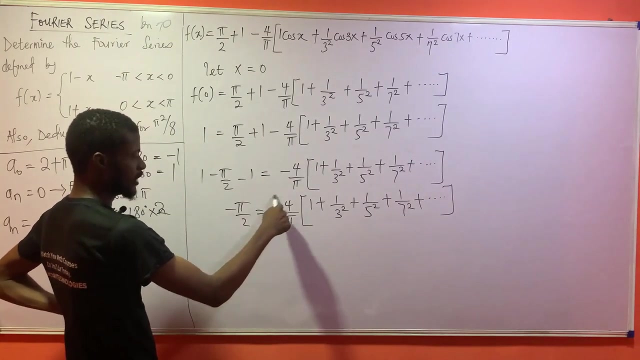 plus. okay, now see, look at this, look at this. we are concerned. we are concerned with pi squared over eight. can i remove everything on this very side? can i remove? because, if you notice, two times four will give me eight, pi times five will give me pi squared. so can i remove everything on this very side? 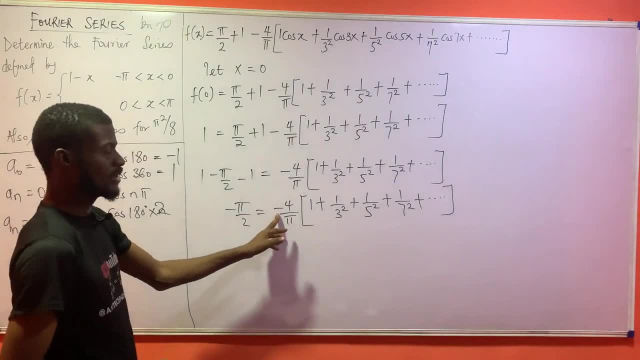 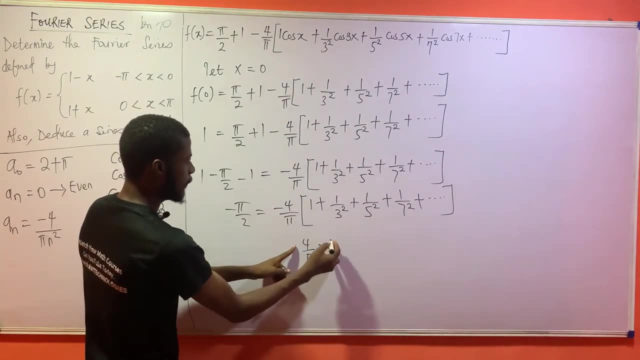 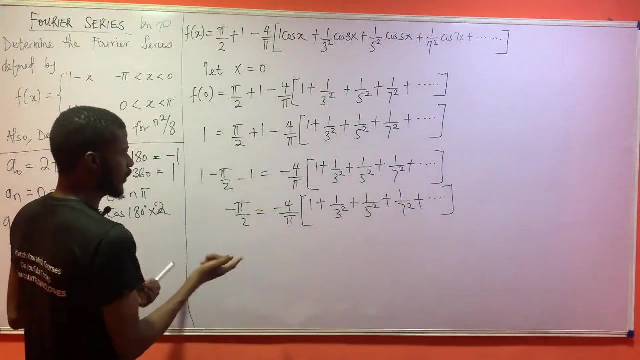 can i remove everything here? yes, can i multiply both sides by pi over four? look at it, i'm trying to remove four over pi. the best way to do that is to multiply by pi over four. i just cannot switch it, just kind of change it over. so, first of all, you agree that minus and minus can take away? 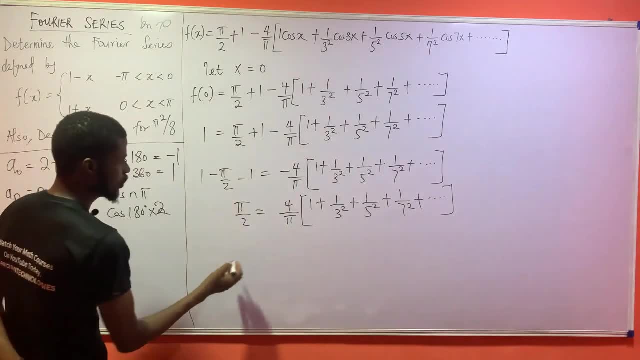 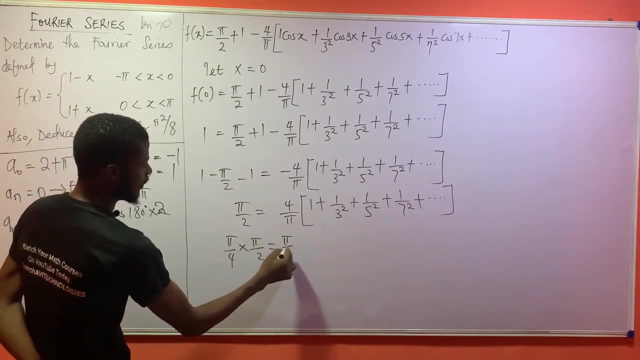 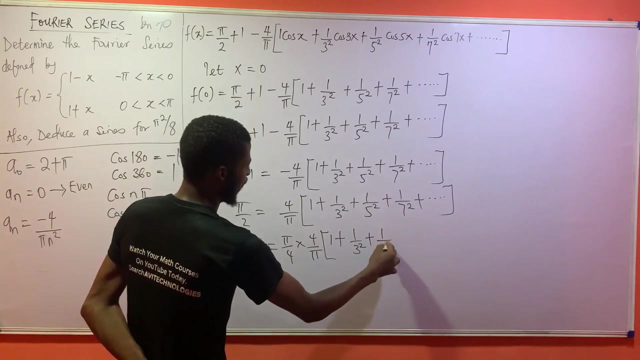 themselves. so let us, let me just remove that they can go away. so i will say: times both sides by pi over four, then times pi over two, equal pi over four times four over pi of one plus one over three, squared plus one over five squared plus one over. 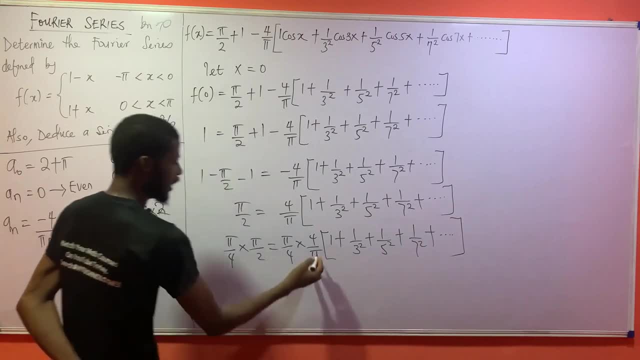 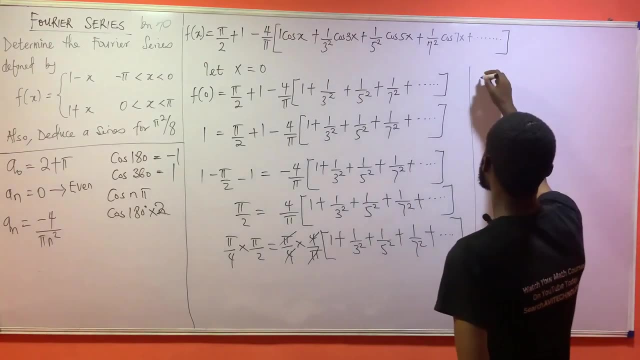 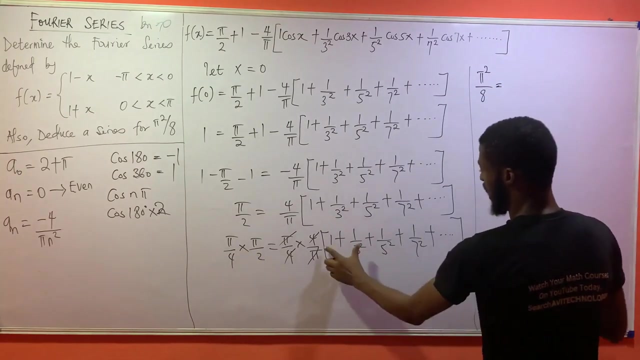 seven squared plus a half. now pi will take away pi four. will take away four pi times pi what i give to us. that will give me pi squared over four times two what i give to me, eight. and all this be equal to everything inside this very place. so this is one plus one over three squared. 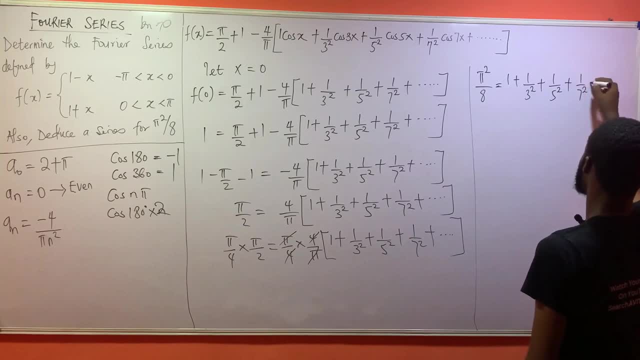 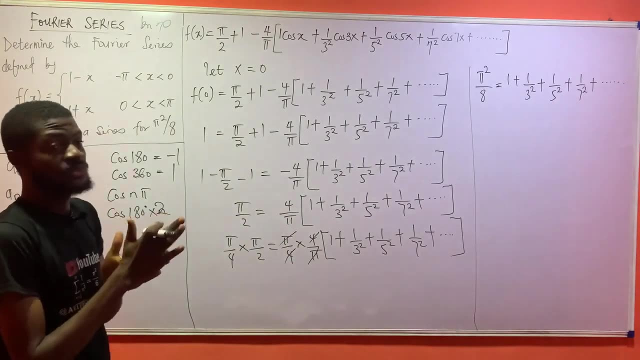 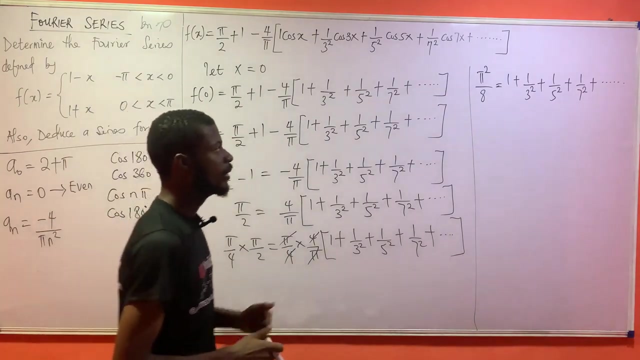 plus one over five squared, plus one over seven squared, plus now. you have deduced a series for that. so that's a series. you have deduced it for that. so this is what you have. this is your final answer, but in a more better form, because this is summation. right, this is summation, i believe. 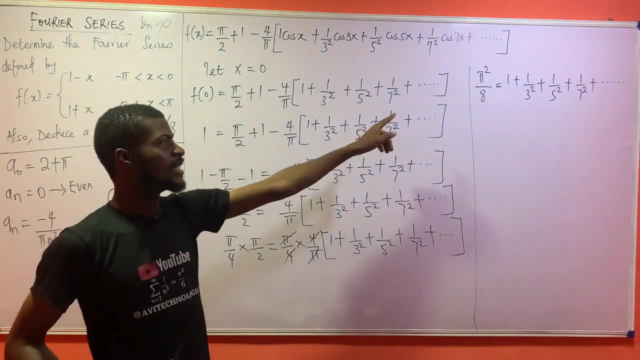 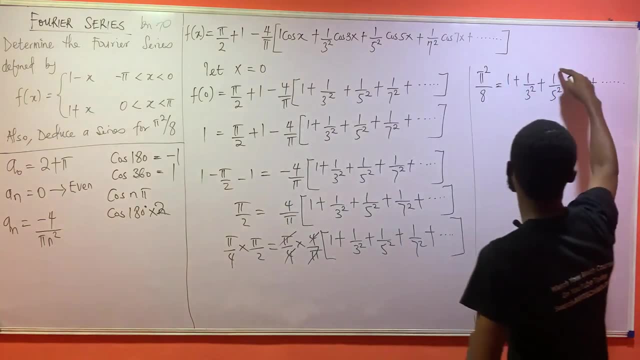 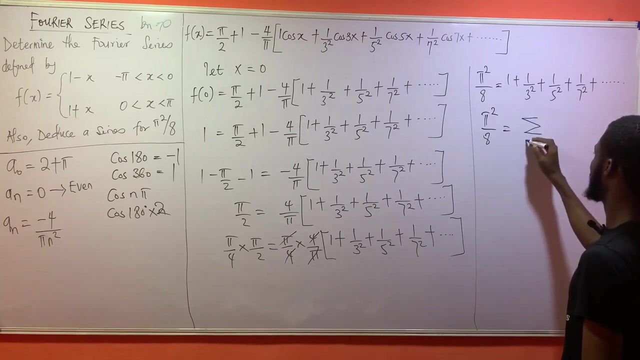 everyone on my show. there's even a summation here. now is there a way we can represent this summation to look like this? it's actually kind of similar. you have one at the top. this is one at the top, one at the top. i would have said that pi squared over eight is equal um. summation from. 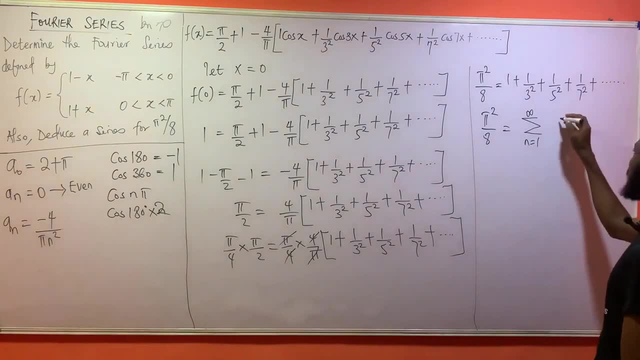 n equal to one to infinity, because we're adding of one over n squared. i would have said so, but if you notice, the formulas are not the same. this one should be pi over six. yes, so the formulas are not the same. why this place? you are only summing with the odd terms. remember, the even terms are: 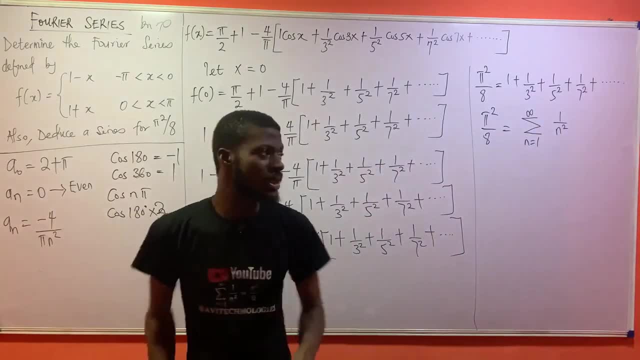 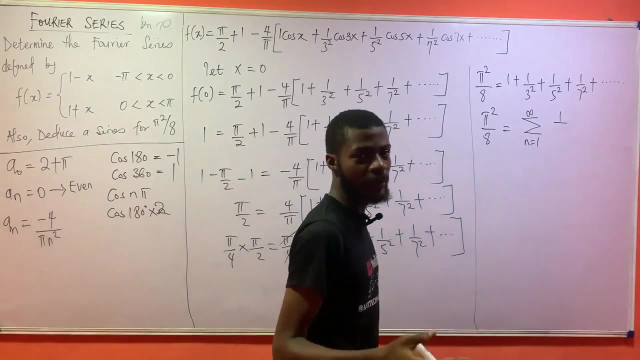 going to give you zero. so you are concerned with the odd terms. so you are going to give you zero terms only. so it means you cannot have n squared here. what am i going to have? i'm going to introduce another variable that is going to be always odd. look at it this way. do you know if i should?